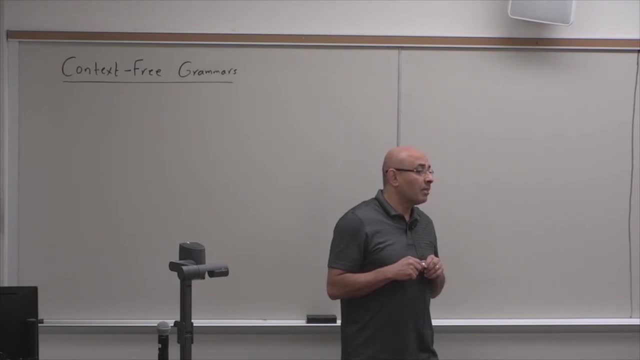 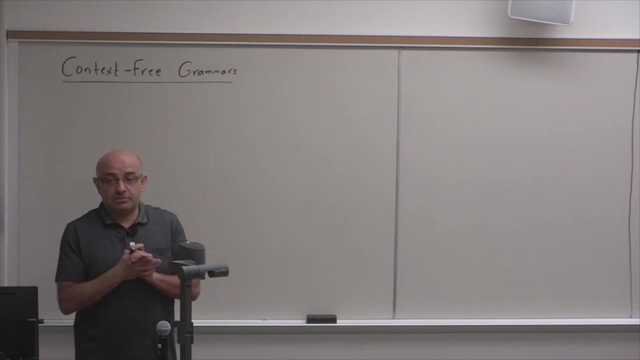 Yeah, There are rules of how to destruct strings, Okay, how to generate strings that belong to a certain language. So basically, you know, informally, it's just a set of rules for defining a language. What kind of language are we talking about here? 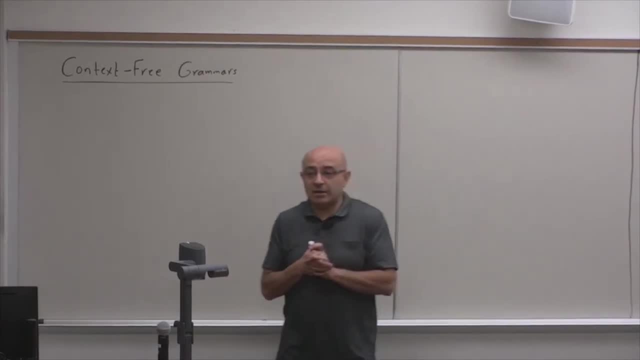 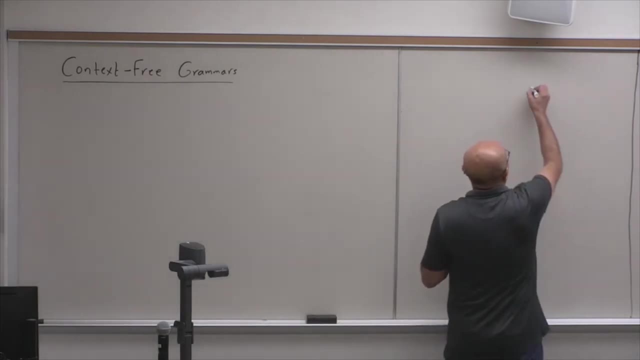 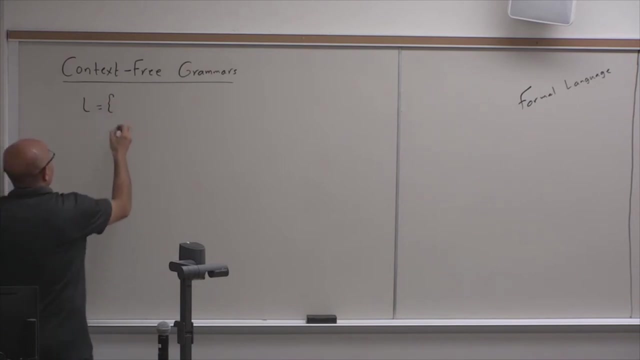 A formal language, right? So we're not talking about a human language or a programming language. We're talking about a formal language Now, the kind of grammars that we defined last time. so we defined a grammar for this language. We started with this language. 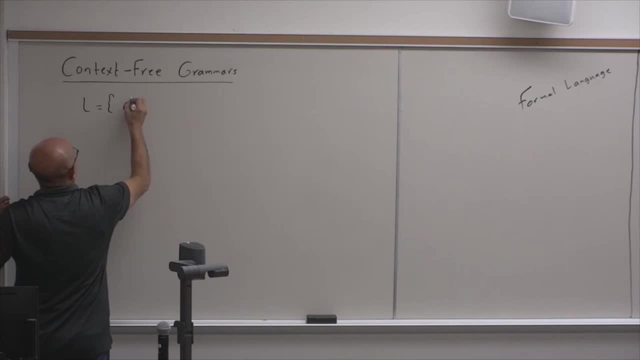 Did I use 01 or A? It doesn't matter. A, A, N, B, N, such that N is greater than or equal to 0.. So we started, we defined a grammar for this language, because this is a language. 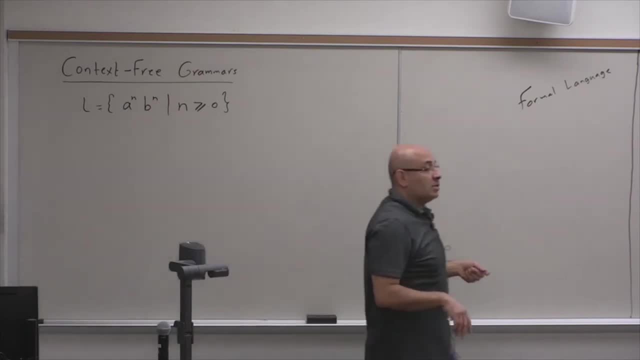 that we could not express using regular expressions, We could not recognize using finite automata because it's a non-regular language And we proved that it's a non-regular language, That it's a non-regular language. In fact, as we will see, grammars can recognize. 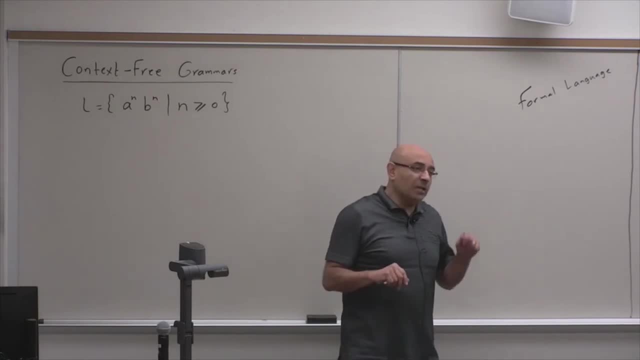 or can generate a larger set of languages, including regular languages. So you can still- as we will see later, you can still- use grammars to generate any regular language. So grammars generate regular languages plus non-regular languages, And I will make this more precise once I define the grammar. 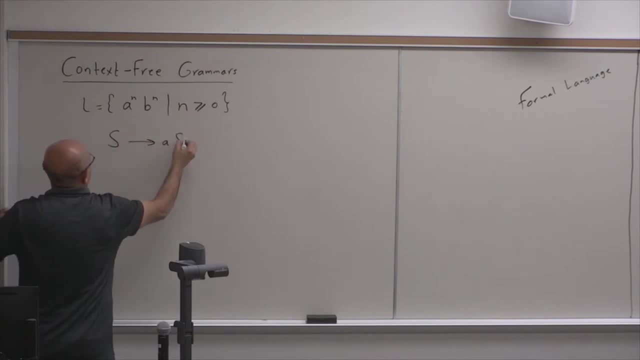 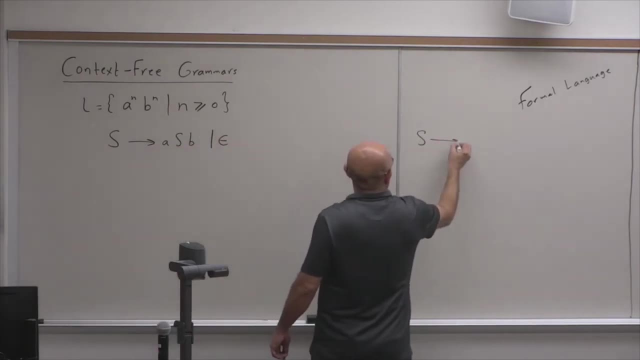 for this. So the grammar is a non-regular language. So the grammar for this is A, S, B or epsilon. By the way, you can write it like this. You can write it: S is A, S, B, S. You can write it. 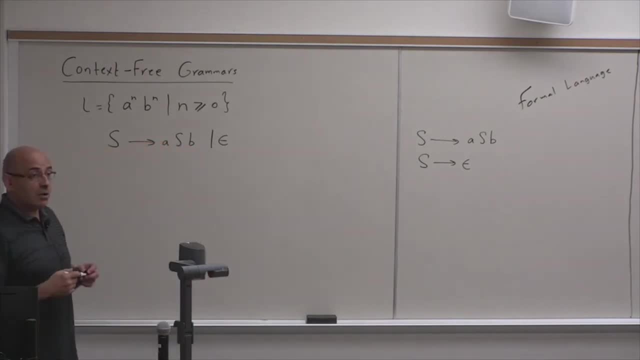 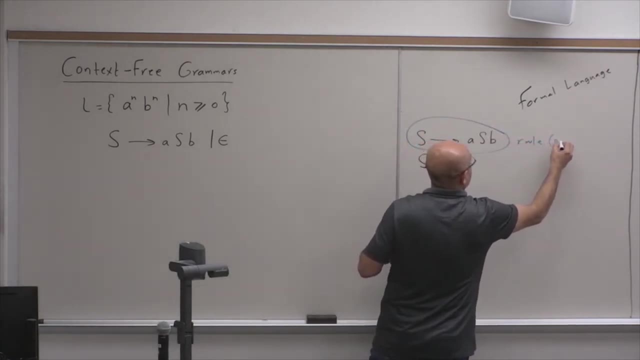 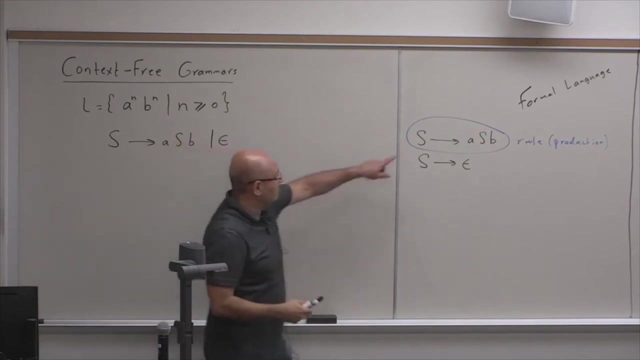 as two separate rules or productions. We call each one of these: this is a rule or a production, And this is a non-regular language, And this is another rule or another production. So you can write them separately, But this is more convenient and more concise. 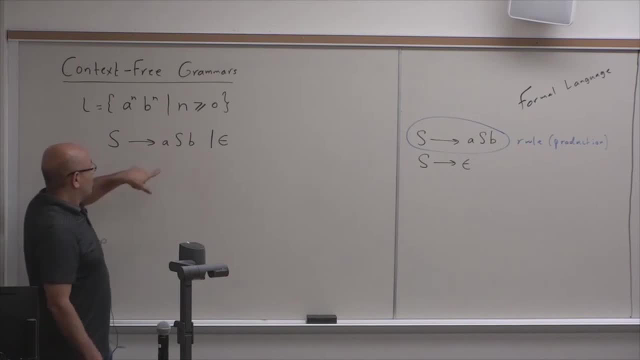 where you write both. you know, because both rules define the same variable or the same, yeah, the same variable. So this is rule number one, This is rule number two. So we just put them together And the relation is or: 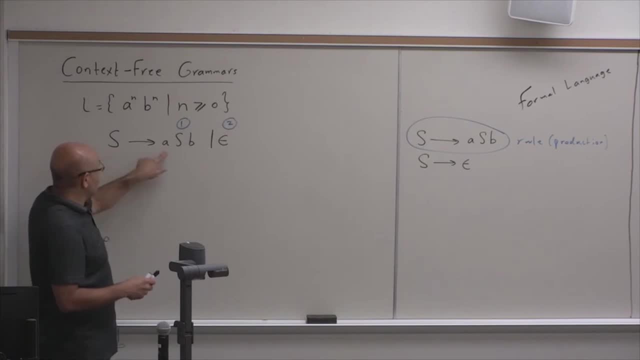 So this is, or So it's just saying S is either A, S, B or epsilon, And this is just another way of saying it, But in both cases each one of these is a separate rule or production. okay, Now, what do I mean by context-free? 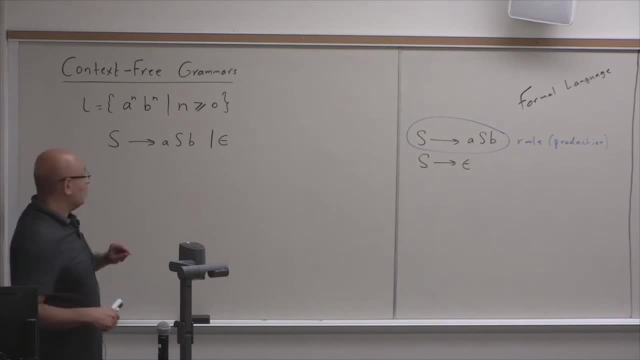 In a context-free grammar, every rule will have only one variable on the left-hand side, And it doesn't have. you know, we have variables and we have what. What did we call these Terminals? Yeah, So like constants. 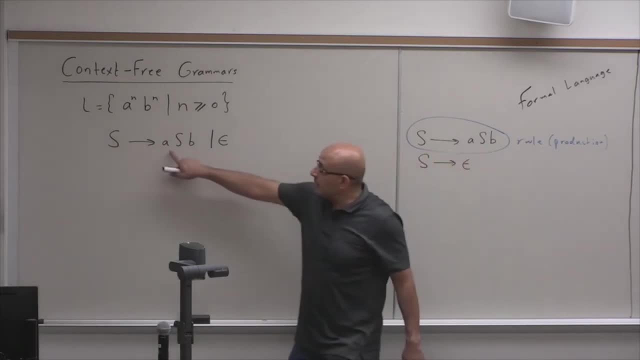 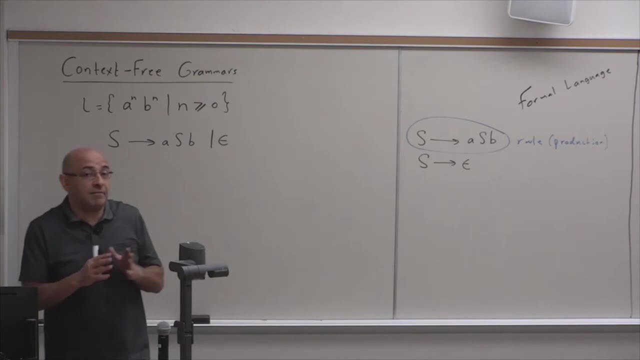 So we have variables and constants. Here we call the constants terminals. So the terminals belong to the alphabet, So the terminals are symbols from the alphabet. So and the- you know, the actual strings that will get generated will consist only of the variables. 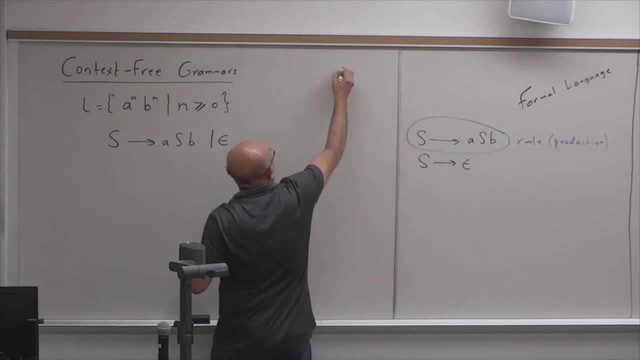 So when you do a derivation, when you do a derivation, you start with S, which is the start variable, And then you derive, you keep substituting And at the end the leaves of the tree should have only terminals. So the root of the tree is. 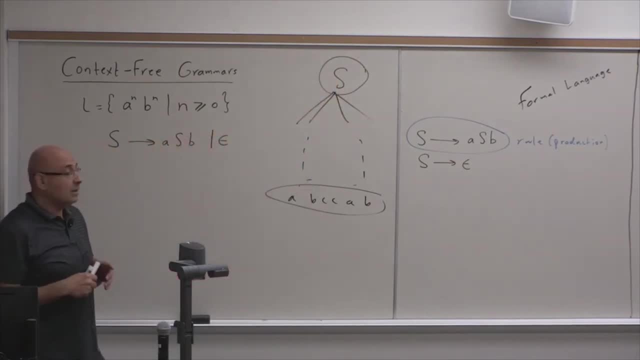 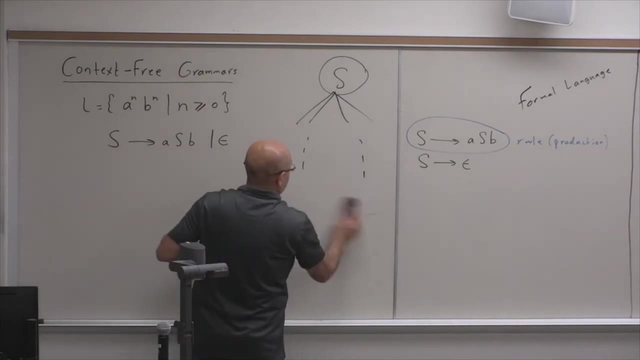 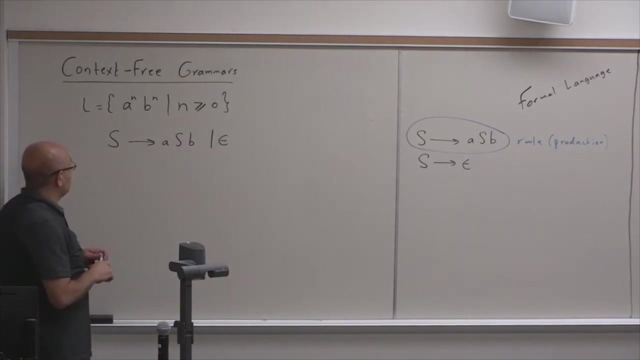 the root of the derivation tree is the start variable And the leaves are terminals. We showed this last time. We can show it again, because this is a new concept for most of you. In fact, how many people have seen grammars before? 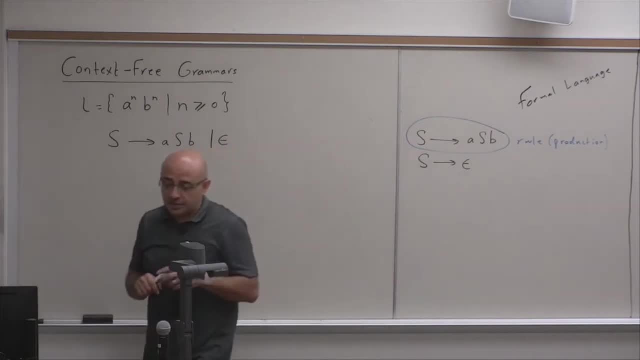 Okay, Only one person. Yeah, Maybe have taken an equivalent class or something. Yeah, But for the vast majority, people have not seen grammars before. Okay, So this is a rule. Okay, So this is a rule. So this is context free. where? on the left-hand side? 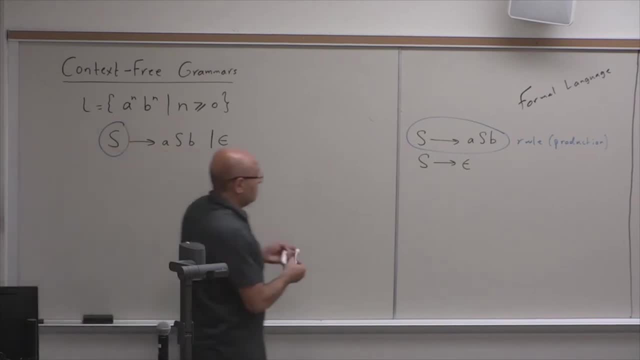 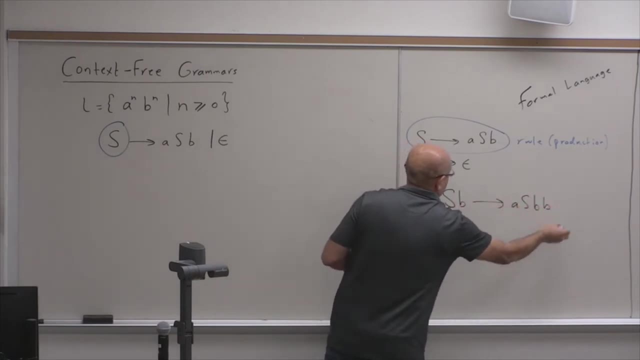 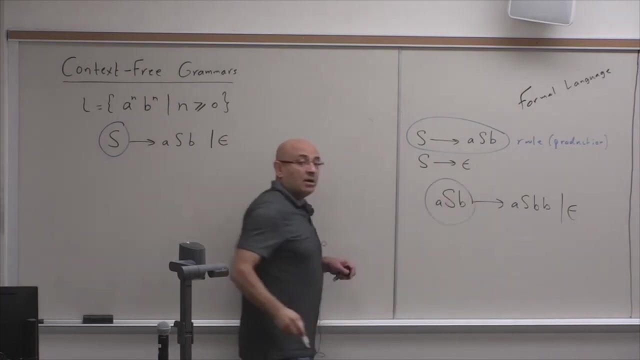 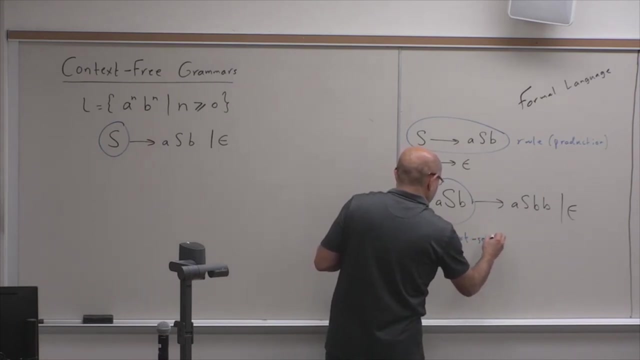 you have a single variable, So this is not context free. So, if you have something like this, This is not a context free grammar. This is a context sensitive grammar. Context sensitive grammar. Okay, So this is a context free grammar. This is a context sensitive grammar. 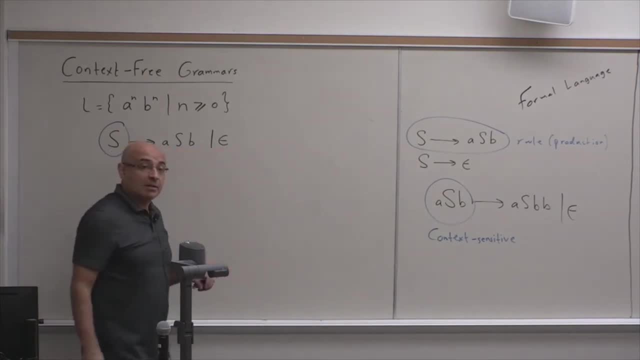 Okay, Context-sensitive grammar. Now in this course we will not deal with context-sensitive grammars. So in this course we will only do context-free grammars where everything on the left-hand side is just a single terminal, single variable or non-terminal. 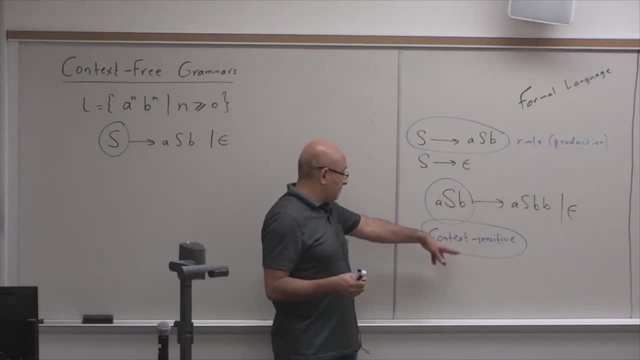 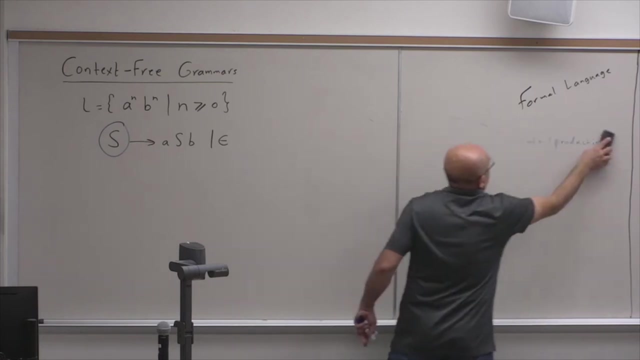 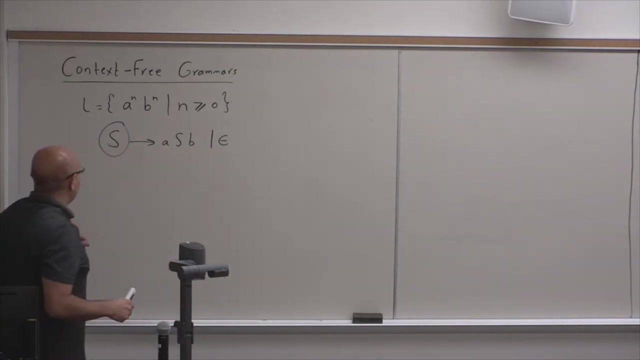 Okay, Just I just want you to be aware of, you know, context-sensitive or grammars that are not context-free. We're only interested in context-free grammars in this course. Okay, And of course, today we'll see more examples of grammars. 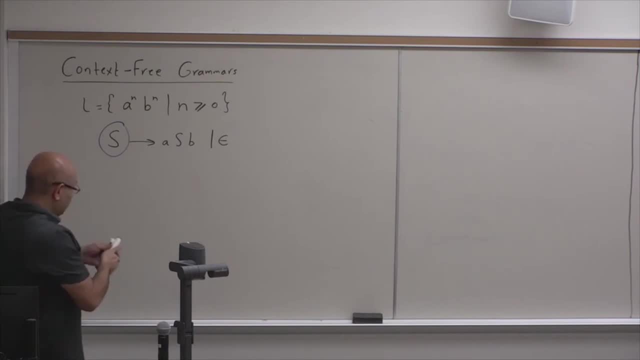 So in this case, let's then write the formal definition of a grammar: So a grammar Or a context-free grammar, Grammar is a quadruple. So the finite automaton was a 5-tuple. This is a quadruple. 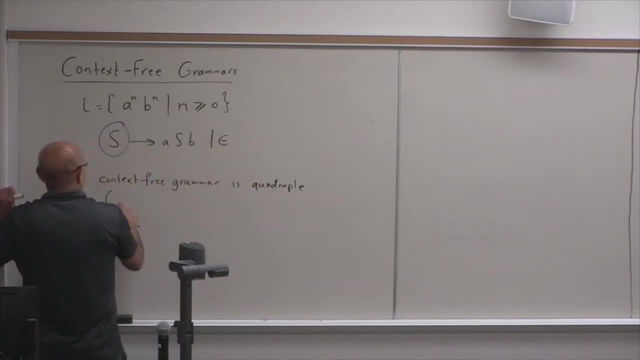 It has now instead of q. what do we have here? So in finite automaton we have a set of states. Here we have a set of variables. Yeah, exactly, Variables are non-terminals. And then we have an alphabet. 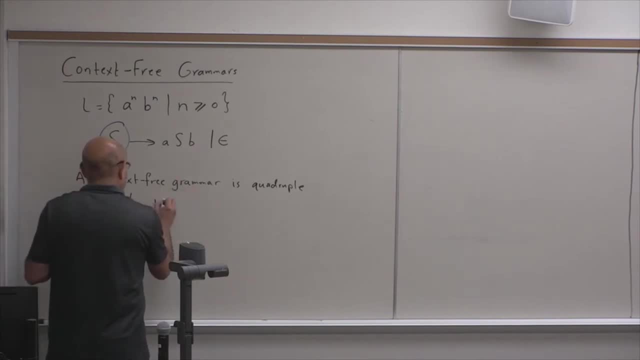 We can call it an alphabet sigma or we can call it a set of terminals. t Same thing. You can also call it sigma. if you want The set of The set of terminals And you have what? Yeah, Can you send the thing that wants to help? 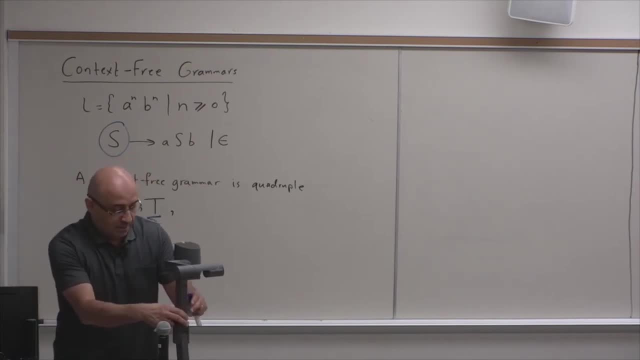 Oh, thank you very much. Yes, Yeah, Okay, There's. I should have a checklist every day to remember to do all the things that I have to do before we start. And I forgot one thing today. Okay, All right. 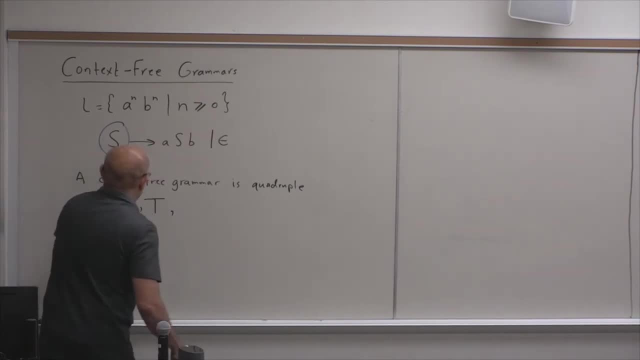 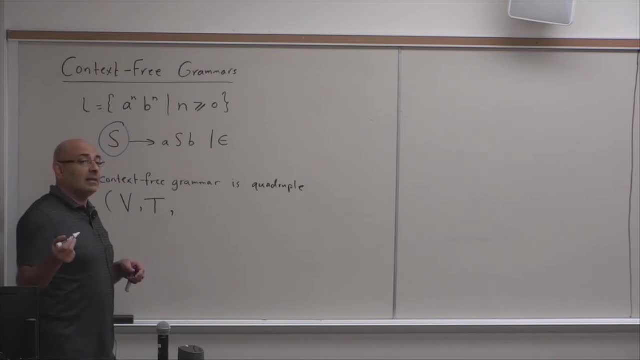 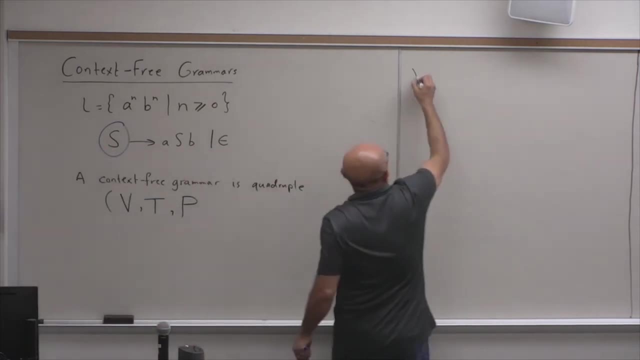 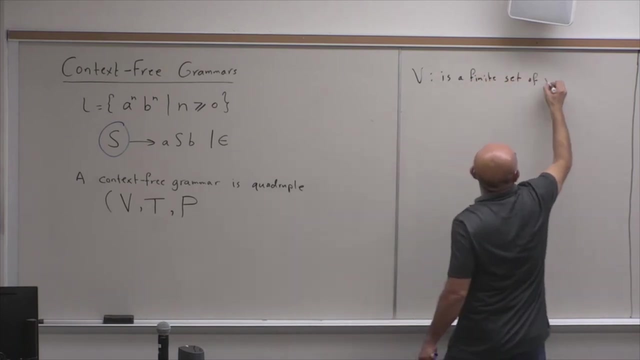 to what in finite automata? The transitions. Yeah, they conceptually correspond to transitions. So this p is a set of, so v, v is a finite set of variables, So we want to yelled a set of foils. 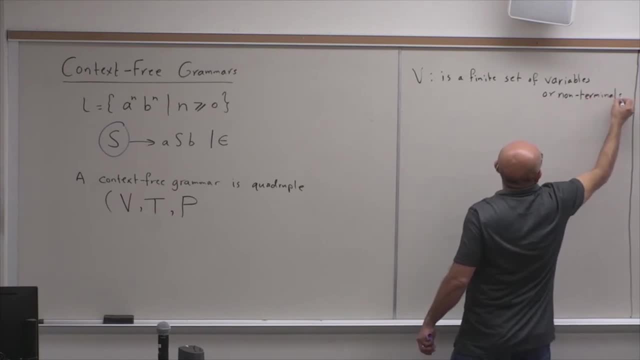 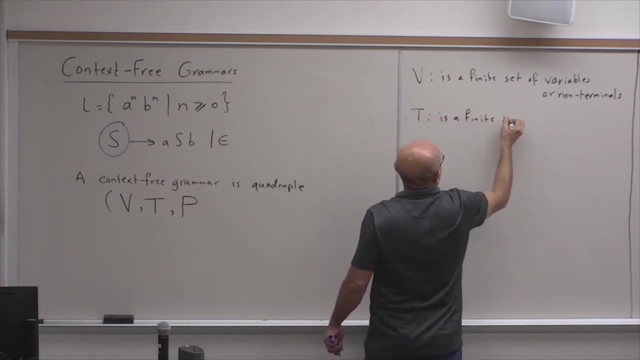 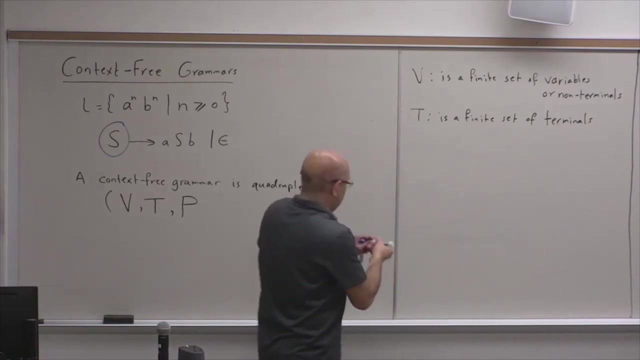 So vie p does thearbife a set of foils. I add different value to the foils: The Las, the v is an infinite set. So we have $$, a dollar, a $$$ dollar out there. So what is that? $$, a dollar, a $$$. 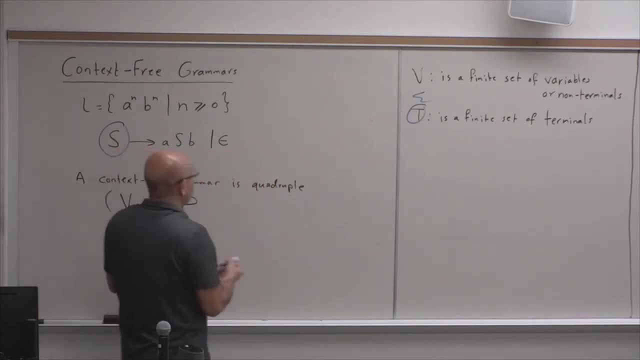 No, no, no. $$ a $$, All right. $$ a dollar a $$ $¦ 1 $$, All right. Okay. So what would it be? What would the $$ a dollar a $$? Ant $觀眾uther suas us. 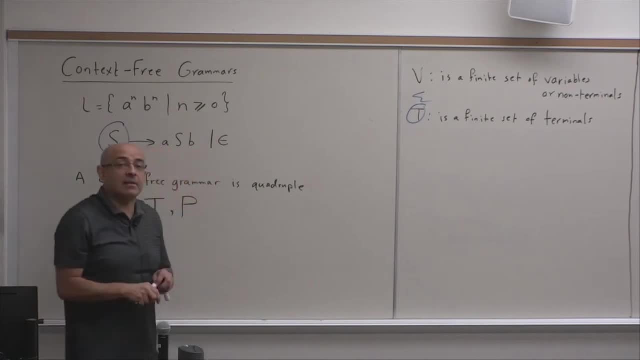 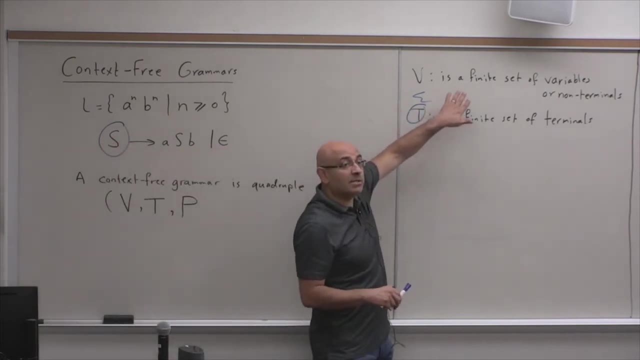 Now, what should the relation between the set V and the set T be? They're both symbols, but what should the relationship be between these two sets of symbols? They should be disjoint sets. You cannot have an intersection. You should use different symbols for terminals and non-terminals. 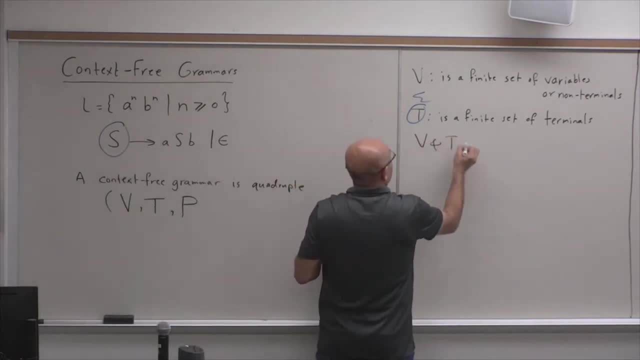 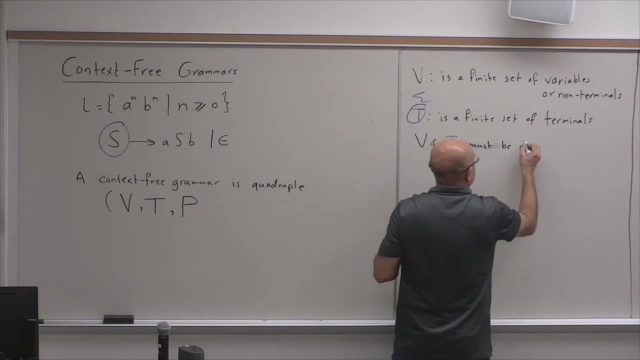 So V and T are or must be disjoint sets. And in our terminology, if you look at this, how are we distinguishing between terminals and non-terminals? How are we ensuring that they're two disjoint sets? Yeah, exactly, We use uppercase for. 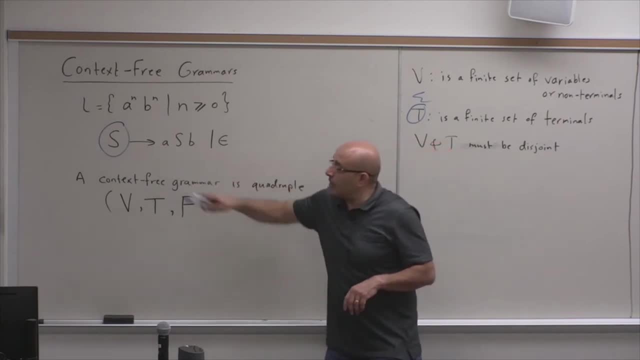 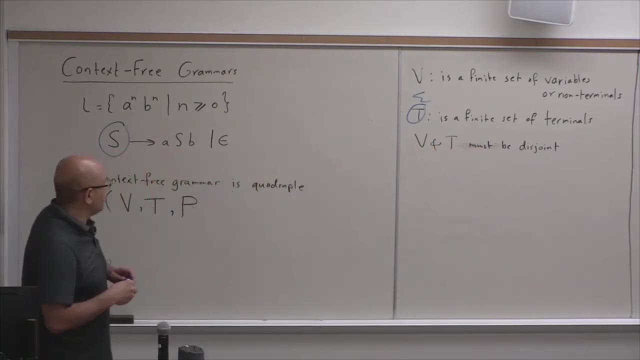 We use uppercase for variables or non-terminals and we use lowercase for terminals. There are other notations that you can see in other books- probably older books, where they underline the terminals. So if you see this with the terminals underlined, it's just another notation or another way. 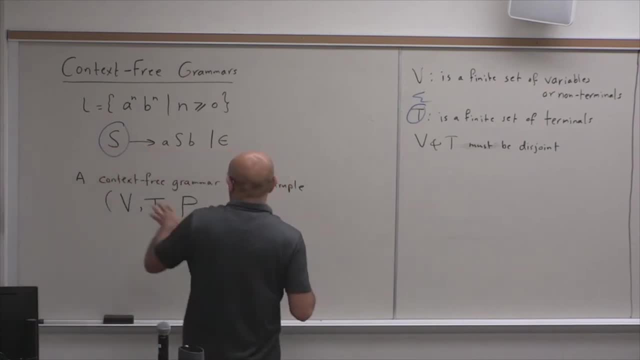 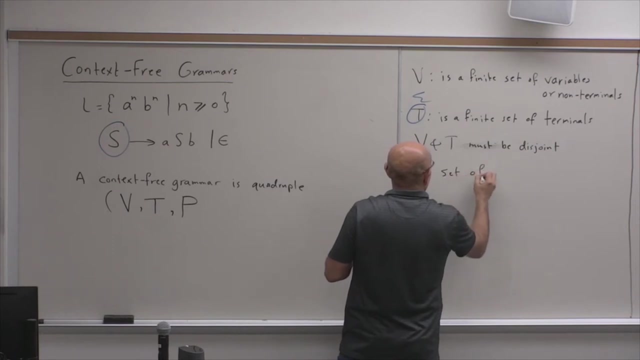 of distinguishing between terminals and non-terminals. I think in our case this is more convenient. So lowercase, Uppercase is a terminal, Uppercase is a variable, And we have P, which is a set of productions. 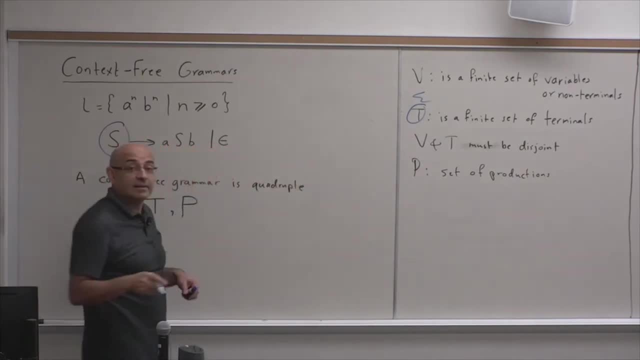 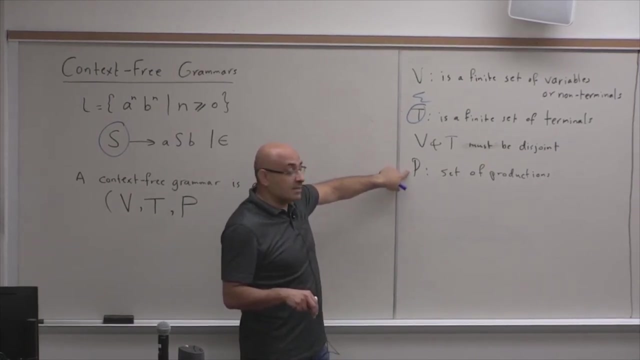 And we have what else? So what did we have in finite automata? So this corresponds to the states, This corresponds to the alphabet, This corresponds to, This corresponds to the transitions. And what else did we have in finite automata? What's that? 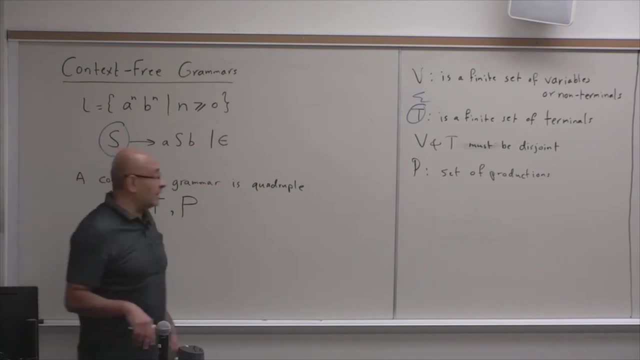 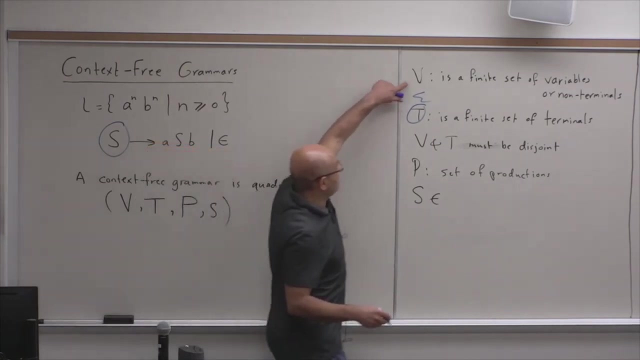 Final states. Final states and start states. yeah, So we have the start variable, S. So S is Here. we call it S the start. Now S must belong to what Which set The set of variables? Yeah, It's a variable. 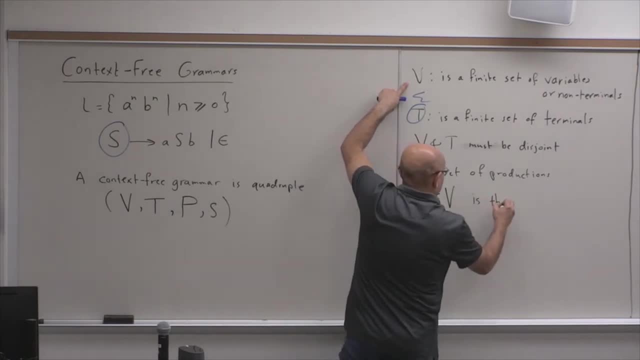 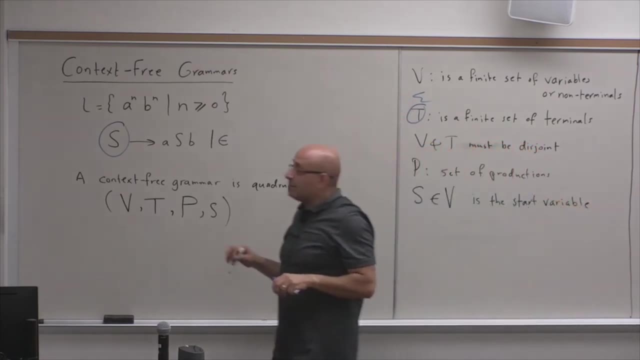 So S belongs to the set of variables Is: Is the set of variables at the start of theissa Yes. Next, which one? The S for the S, The S with the S. Let's define a T, The S with the S in the end of the sentence. 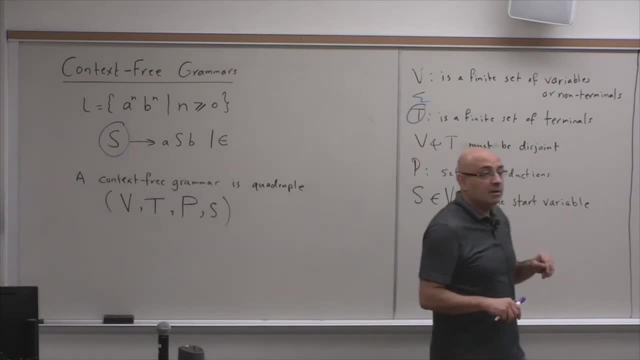 Let's see F. Jinicei is two, Let's see. So that's for there Here. This is a chance forный. Let's use a correct word. Let's use a basic word. Let's use, use T. 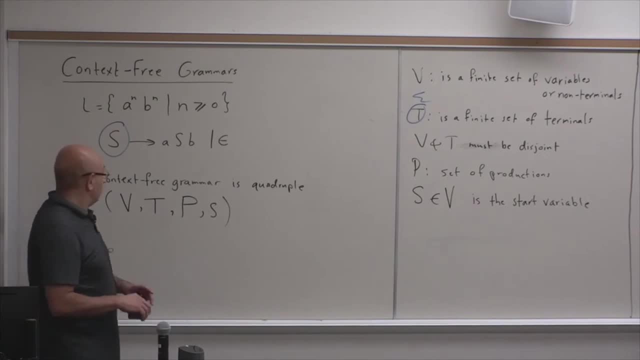 Do you get it? Yes, Now this is what a context-free grammar is. Now the concept of a derivation. A derivation is using a grammar to derive a certain string or generate a certain string. So derive or generate, But in the context of grammars we use the word derive. 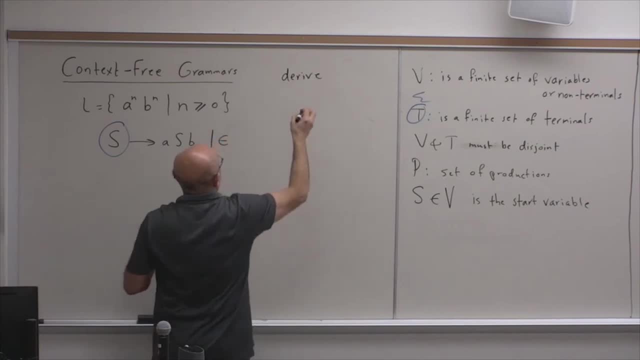 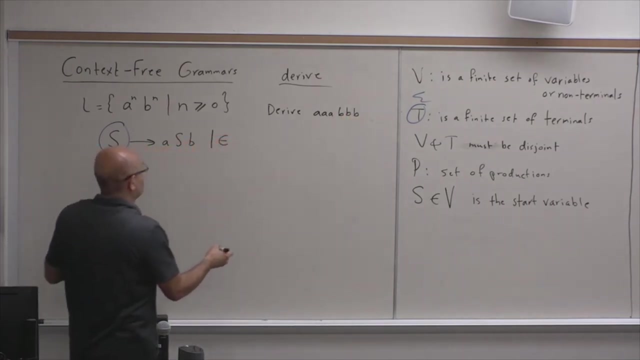 So last time we derived, so let's derive, you know, A, A, A, B, B, B. So deriving A, A, A, B, B, B, we just we start with the start variable. 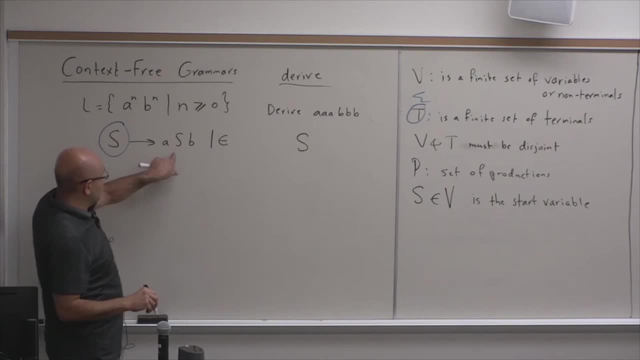 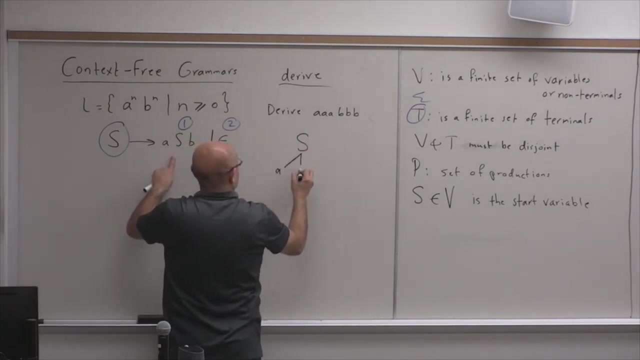 which is the root of the tree. Then we substitute either this or this. So we have two alternatives, or two options, or two productions, Two rules. We pick one of them at a time. So S we substitute. In order to get this, we have to substitute A S, B. Then 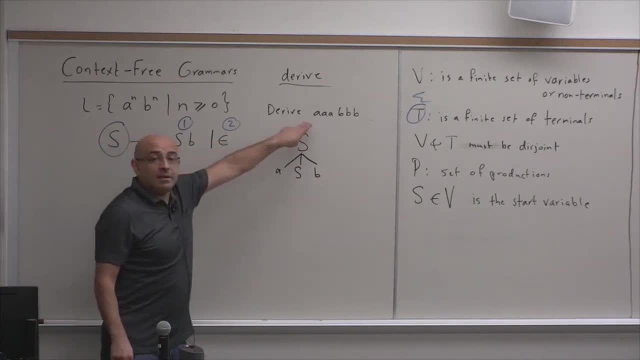 we should repeat this three times in order to get three As. So again we substitute for S A S B, And again we substitute A S B, And the final substitution is epsilon. Yeah, And of course you know, for, in order for a definition. 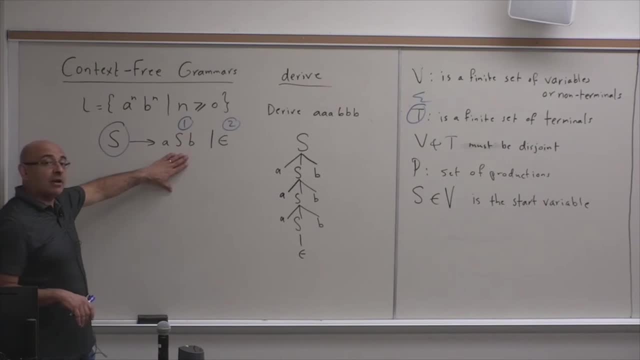 to make sense. well, this is a recursive definition, right? What do we mean by recursive here? Yeah, So it's defined in terms of itself. We are defining S in terms of S, So S appears on the left-hand side and on the right-hand side. 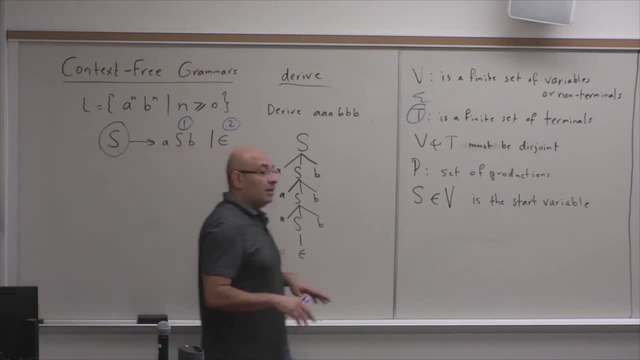 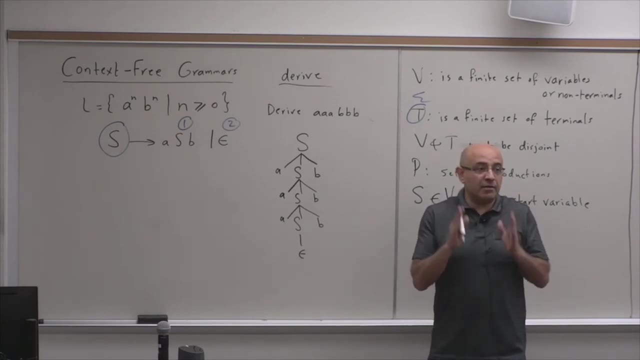 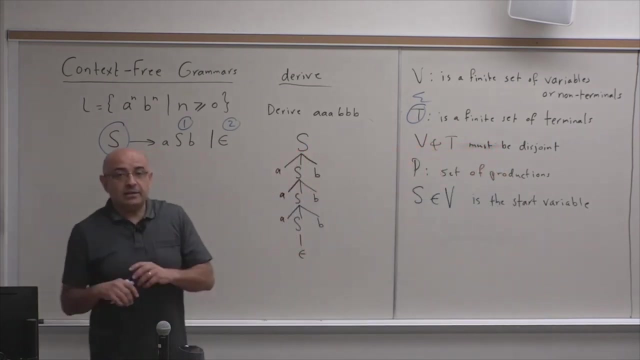 So this is a recursive definition, And in order for a recursive definition to make sense, it has to have what In addition to the recursive definition? Yes, Yes, In addition to the recursive rule, you have to have a direct rule that defines the variable directly, not in terms of itself. 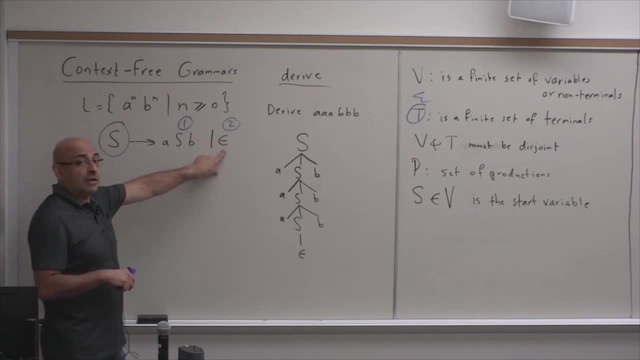 So we have to have this direct rule or base for the recursion, And this is the recursive part of the definition. Derivation can be done using this derivation tree. Okay, So this is the derivation tree, So we can do the derivation textually. 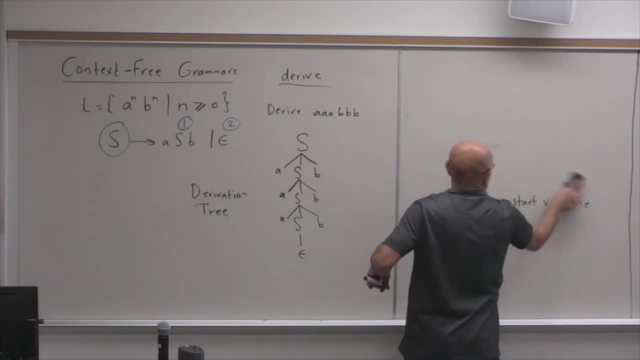 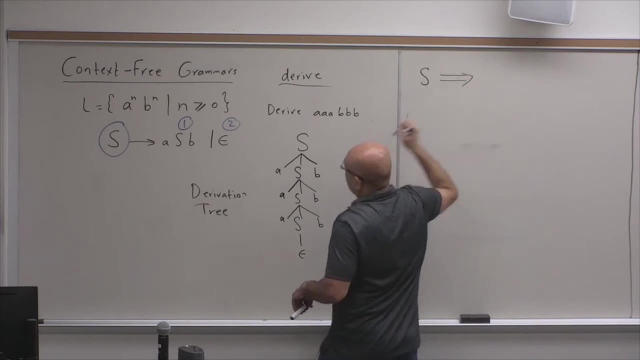 We can do it just: we say: okay, we start with S. Then we say: by rule number 1, we substitute ASB for S, So S expands into ASB. Or let me write it: Okay, Let me write it here. 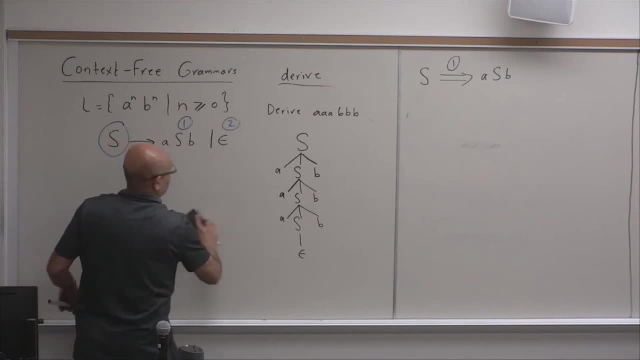 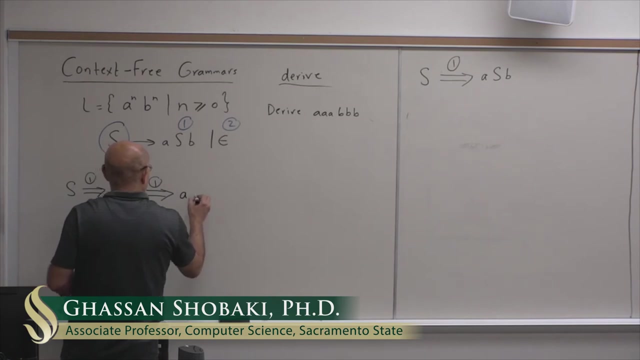 I think I will have more space here. I don't want it to be on. Okay, So S using rule 1, we get ASB. Then we use rule 1 again to expand this S into another ASB, So we get AASBB. 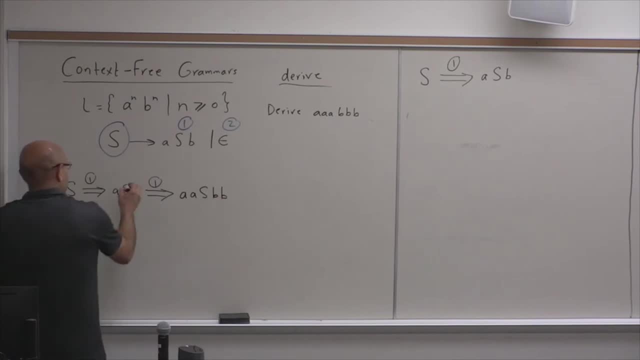 So, by the way, I'm going to write it as ASB. So basically, this rule expands this S into ASB or substitutes ASB for S using rule number 1.. So these are just substitution rules. So then do we apply it again. 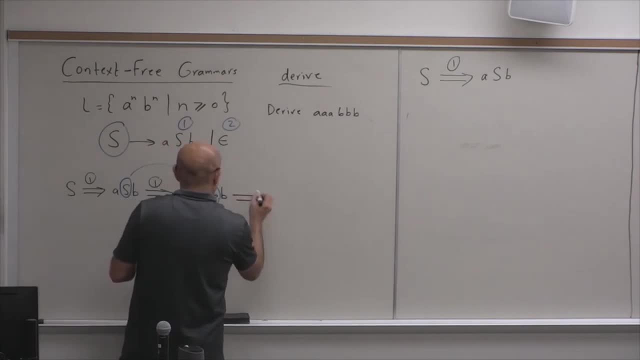 Yeah, We apply it one more time Again, using rule number 1, we substitute now ASB for this S, So we do A, A, A, S, B, B, B And again, what we are doing here is substituting for this S ASB. 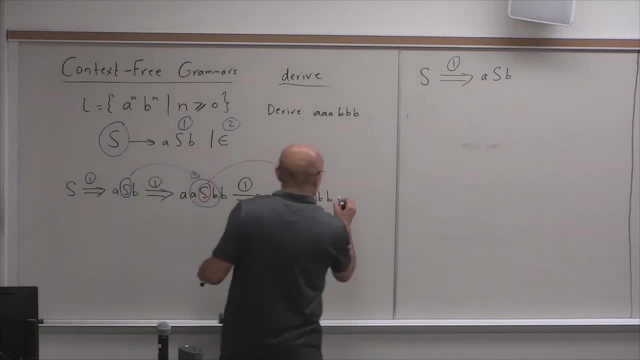 Okay, And the final substitution is using rule which rule? Rule number 1.. Finally, we use rule number 2.. To substitute an epsilon for S, you can write an epsilon or just drop it, because it's epsilon, the empty string. 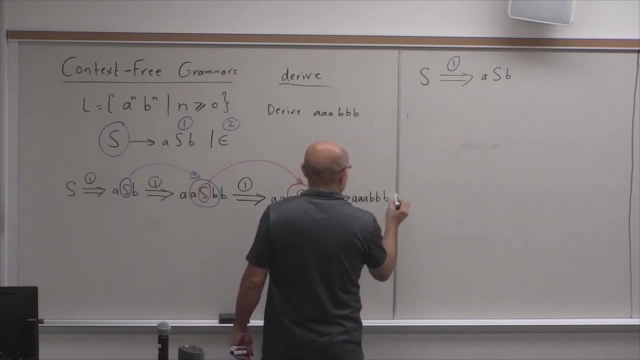 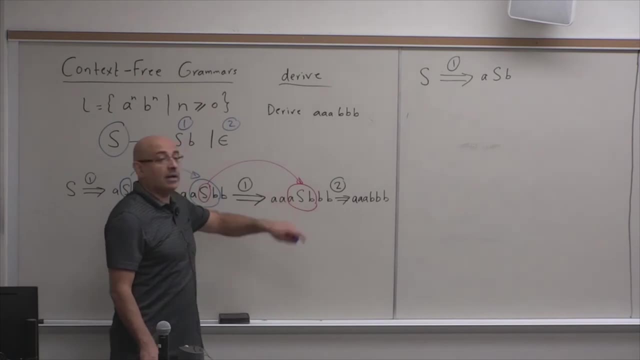 So you can just say A, A, A, B, B, B. Normally we don't write the epsilon, So it's like you are substituting nothing for S. Okay, So this is a derivation, So there are two different methods of representing S. 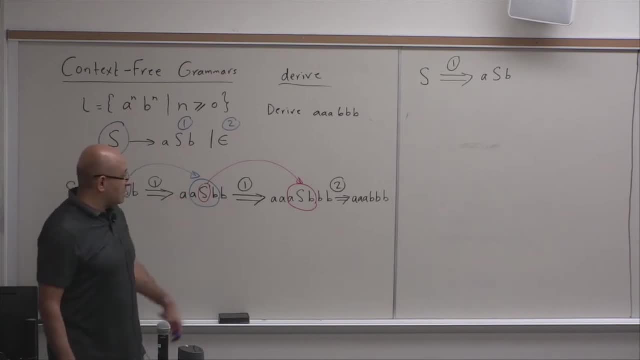 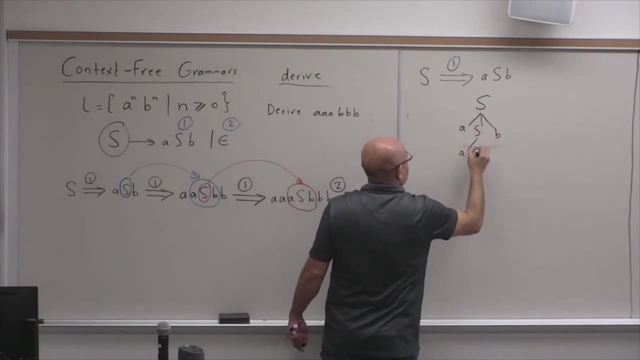 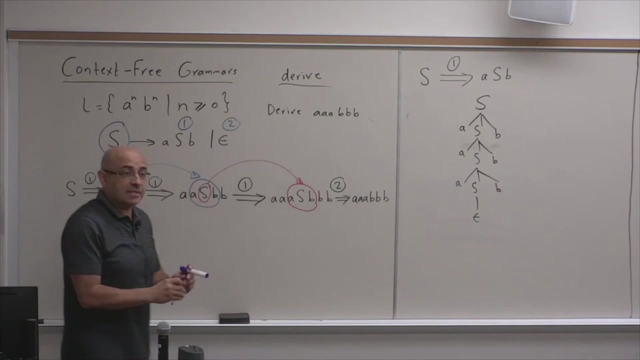 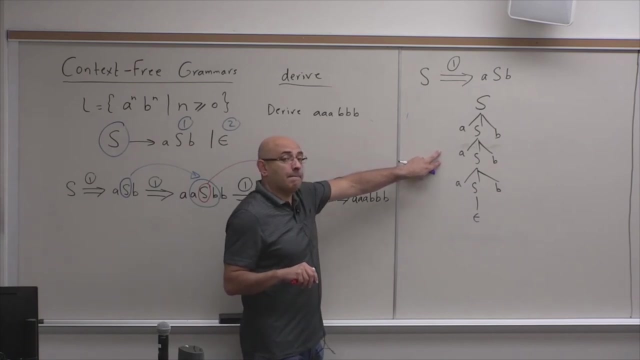 So this is a derivation, either this textual method or the tree. And when you read the string that you derive, you read: how do you read it in the tree? How do you read the derived string Left to right, you read what? 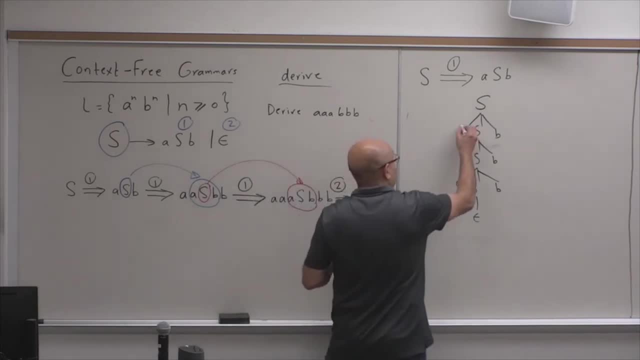 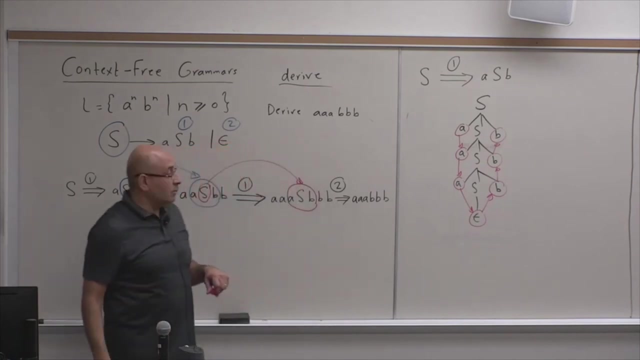 The leaves. You read the leaves left to right. Leaf, leaf, leaf. So it's like this: This is how you read the string. You read the string. You read the leaves left to right And, of course, for a complete derivation: 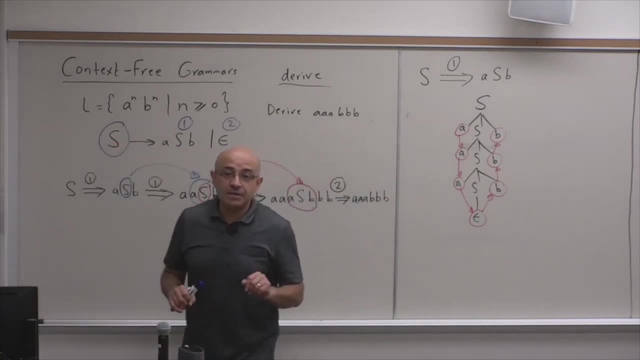 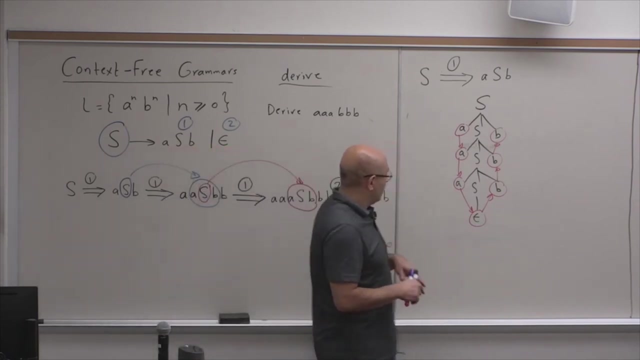 in a complete derivation all of your leaves must be terminals. So when some of your leaves are straight, some of your leaves are still not terminal. you don't have a complete derivation yet You are in the middle of a derivation. So if at some point you know you don't have a like this, 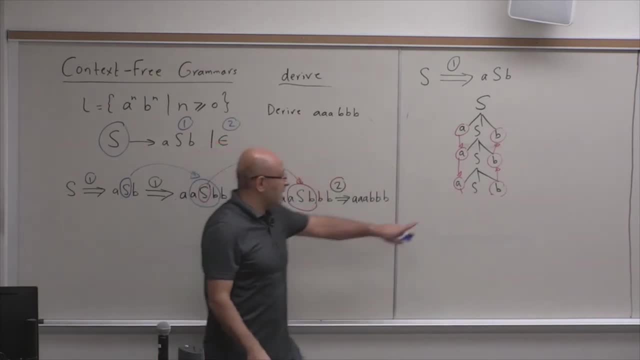 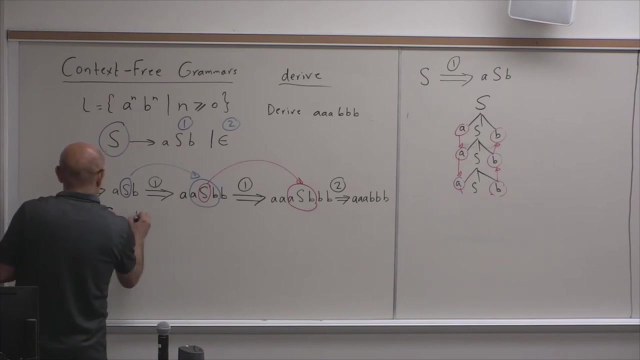 This is an incomplete derivation because you still have a leaf that is not a terminal. Okay, So in this case we say that you know S derives A, A, A, B, B, B. Or we can say S star A, A, A, B, B, B. 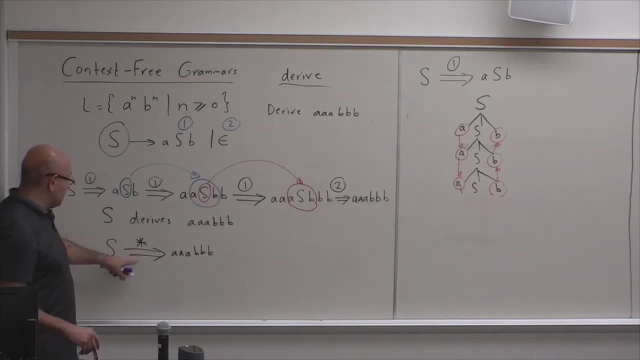 So this notation here means that S derives A, A, B, B, But the star means that this: there can be multiple steps that lead from S to A, A to this string, And these are the steps. So you use this for a single substitution. 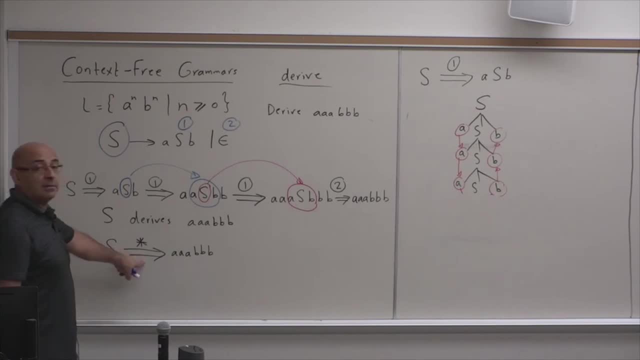 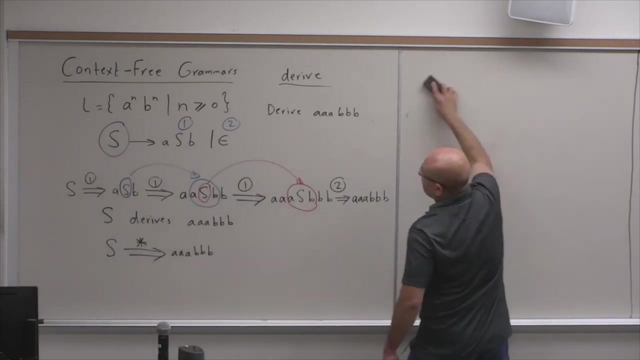 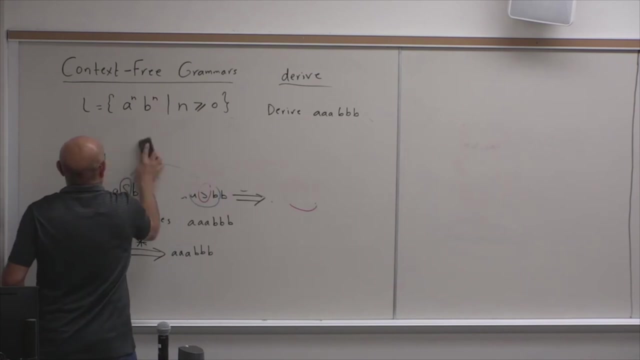 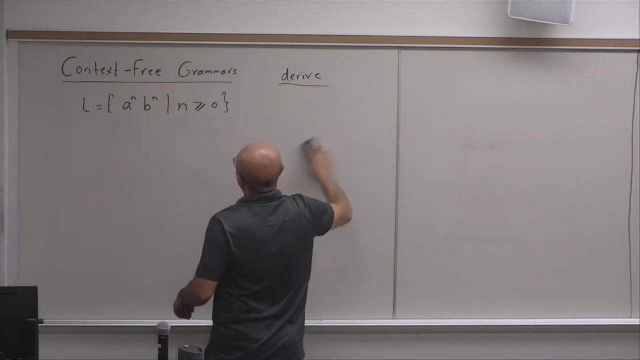 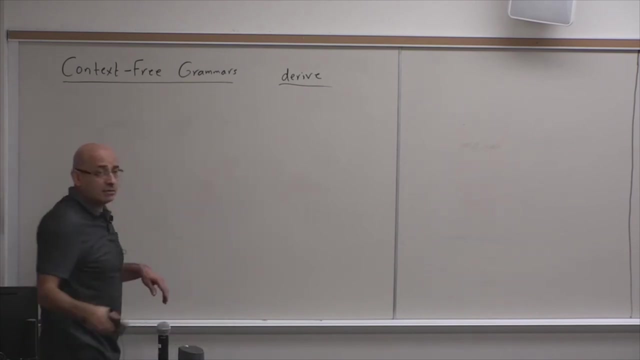 You use this to abstract multiple substitutions. You can go from S to A, A, B, B, B, Okay, So let's take another example. Okay, Well, let me write a grammar and then let's figure out the language. 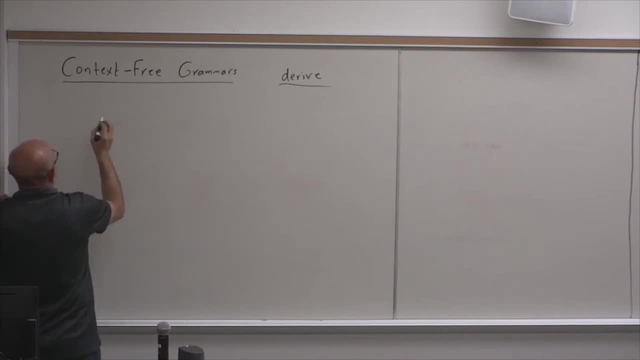 What does this language generate, Or what does this grammar S is A, S A Or B, S B Or epsilon. Okay, Now, how many? how many productions do we have Three? We have three productions. 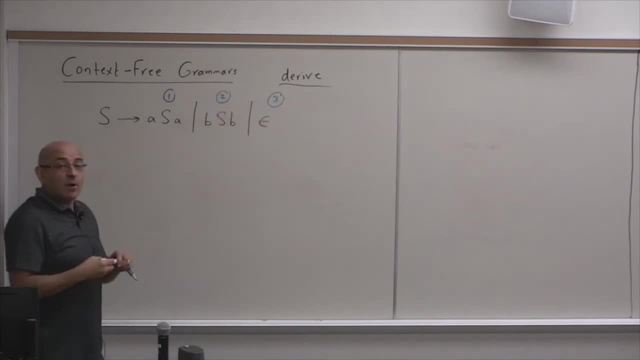 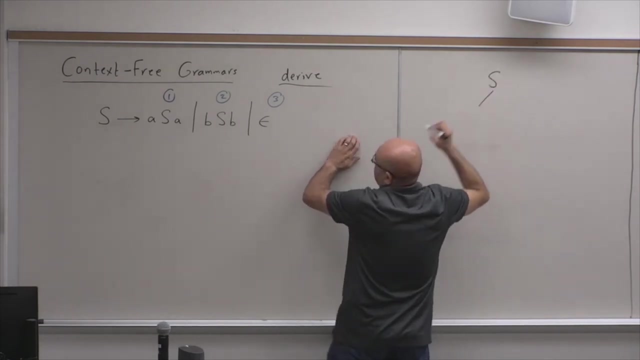 Or rules. Now, what does this? what language does this grammar generate? Well, let's try to do something. We have some derivations. So what if I do this S I can substitute A S A. So let me substitute A S A. 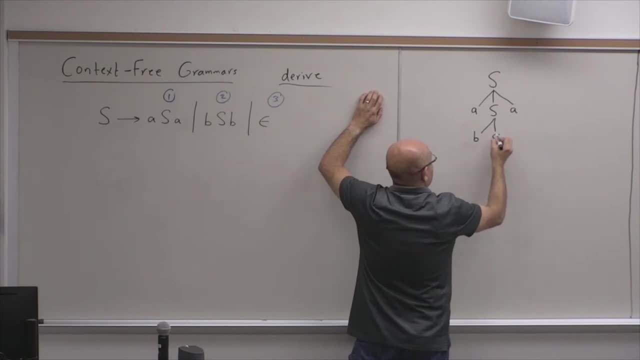 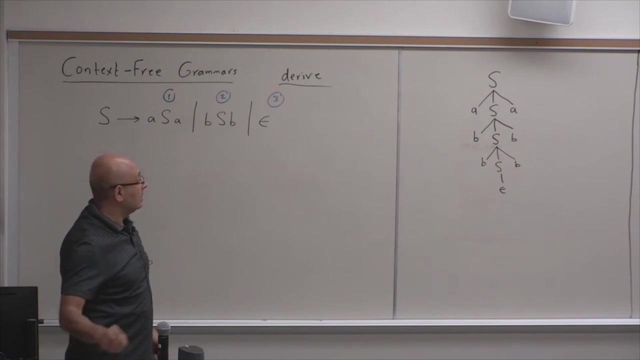 Then let me try to substitute B S B. Then I can substitute either A S A or B S B or epsilon. Let me substitute B S B. again. Let me substitute epsilon. What's the string that gets generated here? 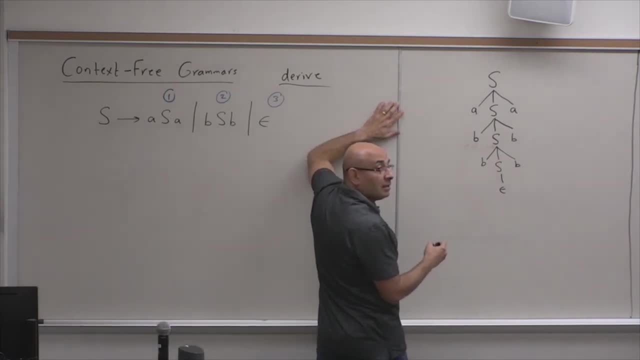 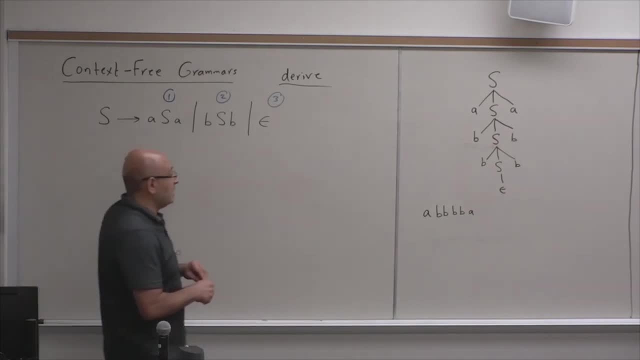 I mean what? What property do all the strings that are derived using this grammar have? Well, this is one property. yes, They will always have an even number of A's and B's, That's true, But that's not all. 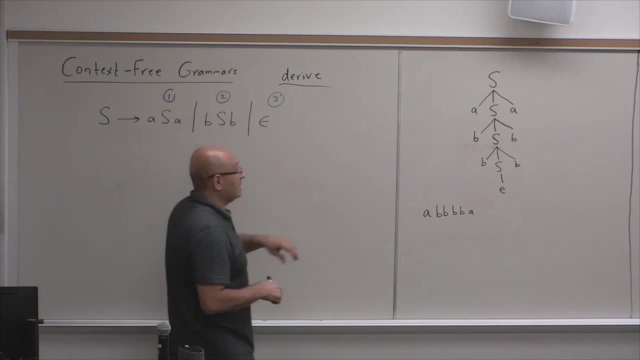 That's not, you know. it doesn't generate all the strings that have an even number of A's and B's. It generates something more specific than just an even A's, an even number of A's and an even number of B's. 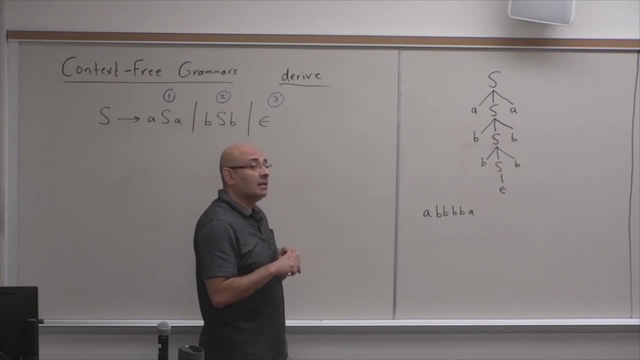 Yes, Does it start and end on the same character. What's that? Well, again, it starts and ends with the same character. Yes, that's true, But it's more specific. So this is not that's true. 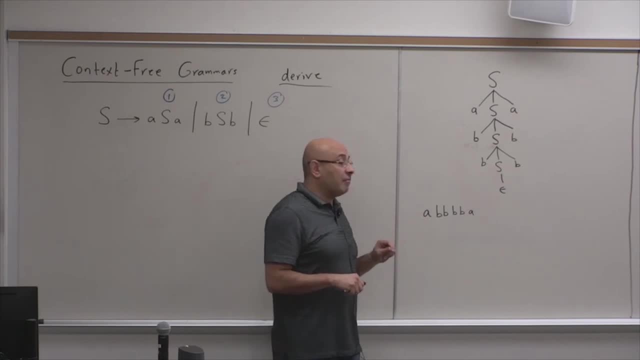 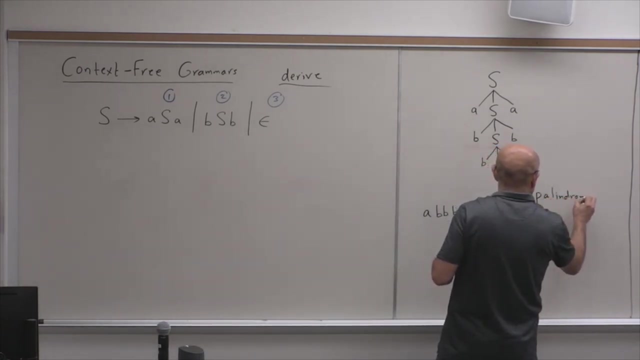 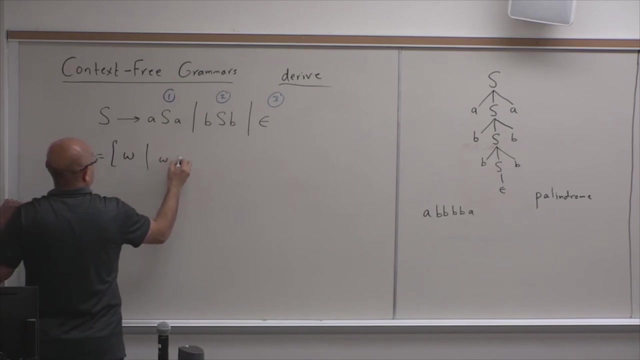 But the strings that belong to this language have a more specific and a stronger property. Yes, A palindrome? Yeah, exactly, So this generates palindromes, Cool. So this is the language here. W is the set of strings W, such that W is a. 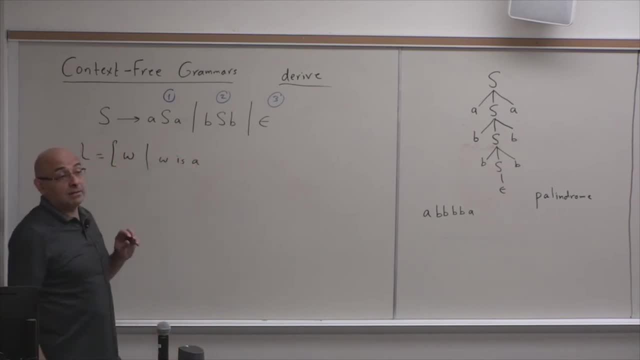 Well, but does it generate all palindromes? What kind of palindromes does it generate? So it doesn't generate all palindromes. So this is a palindrome here. ABA, Does it generate this? Yes, 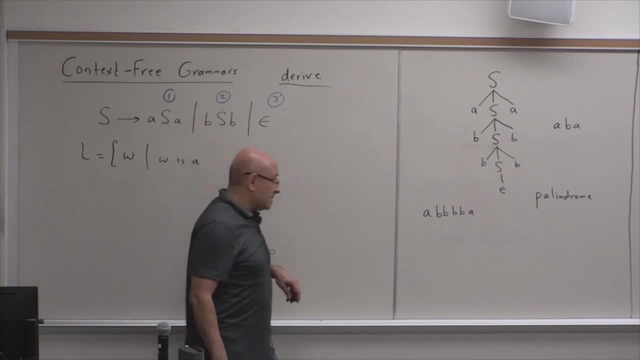 Okay, So it's. yeah, it generates even length palindromes, So is an even length palindrome, And an even length palindrome is. you can also Describe it, as you know. you can split it in half. 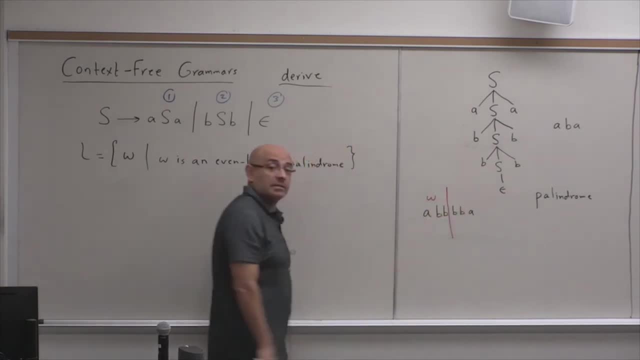 And if this is W, what can you say about this? WR? WR, the reverse. Yeah, You can write it L. Another way of writing this is the set of strings WWR, such that W belongs to sigma star or T star. 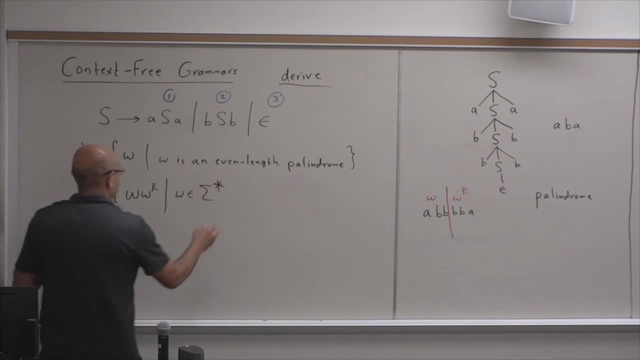 Whether you call the set of terminals sigma or T. Here we are calling the set of terminals sigma, So it's WWR. Okay. Now the next question is: how do we modify this grammar to generate all palindromes? 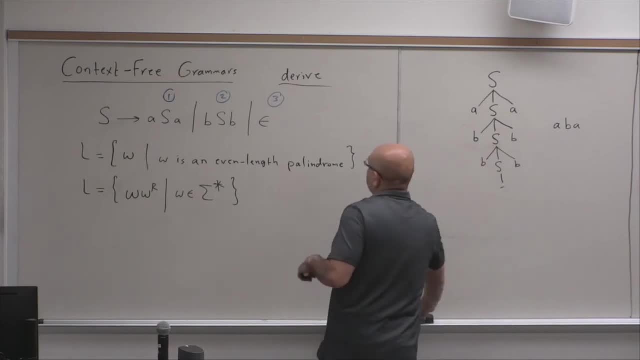 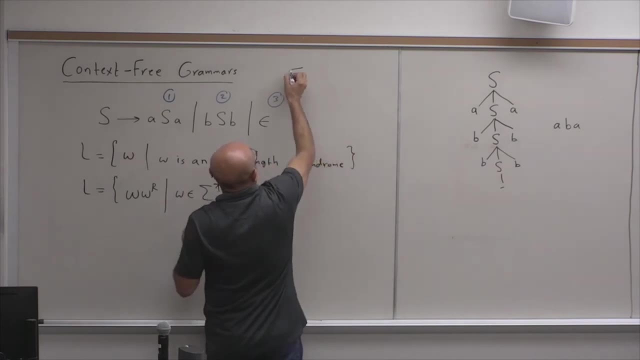 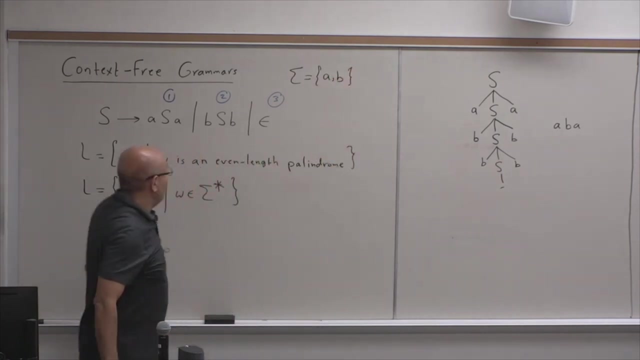 Not only, Not only even length palindromes. And of course, our alphabet- let's write it explicitly- is AB. On this alphabet, how do we modify this grammar such that it generates all kinds of palindromes? 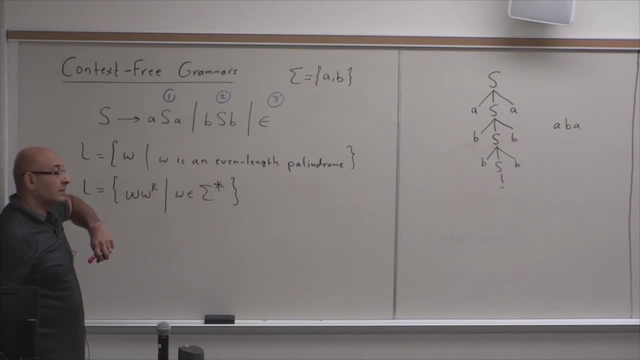 Yes, You change to. so it's just BS or SB, BS, or what do you mean BS? So You would just, instead of having two B's, you would just take one out. No, this is not going to do it. 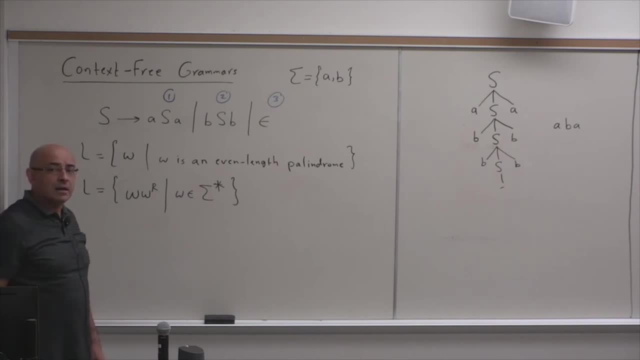 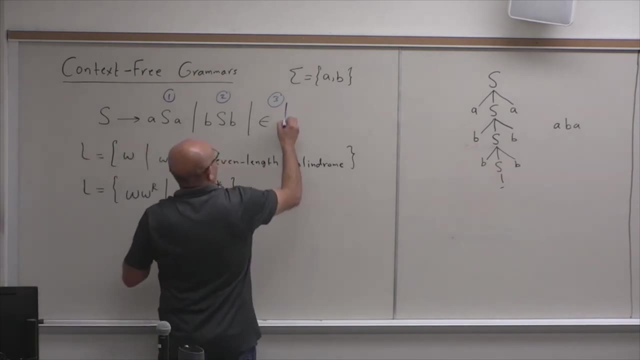 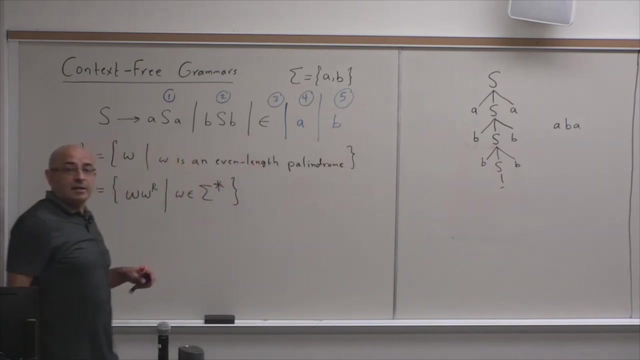 Yeah, You just put A and B as the other terminal. Yeah, exactly. So if you do this, Okay, If you add rule number four A, rule number five B, then this will generate all you know even and odd length palindromes. 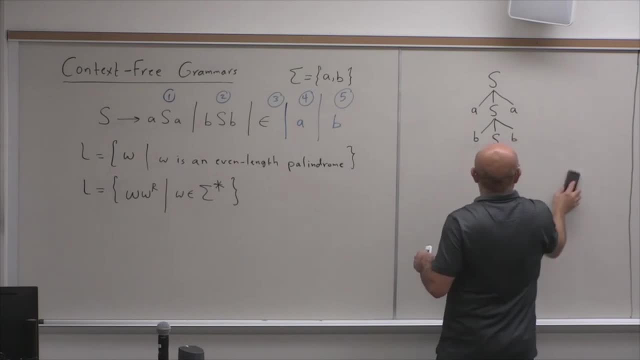 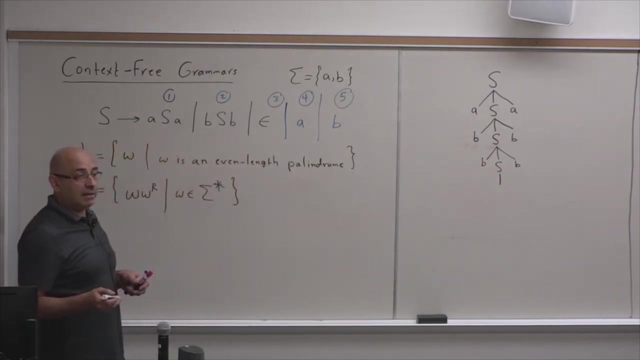 So to make sure that we verify this, so we can say ASA, BSB, BSB, and then you know we can substitute for S What We can have. if we put an epsilon, we'll get an even length. 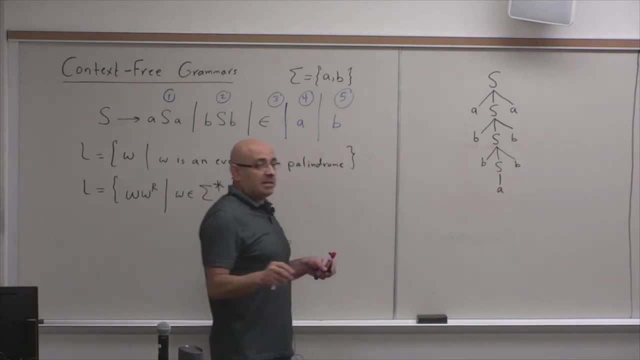 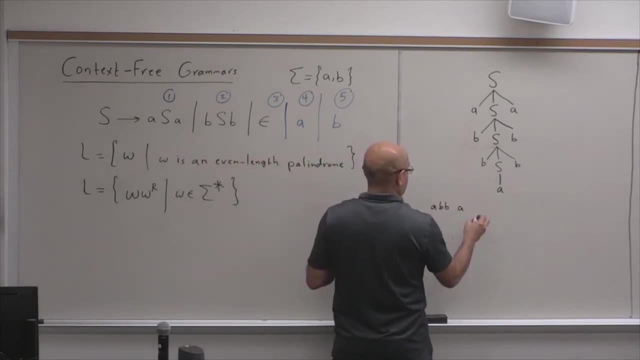 If we put an A, you know this is going to be the symbol in the middle. So this is going to give us what: ABBA. I just put this space so that we can read it: ABBA. So you have your something in the middle. 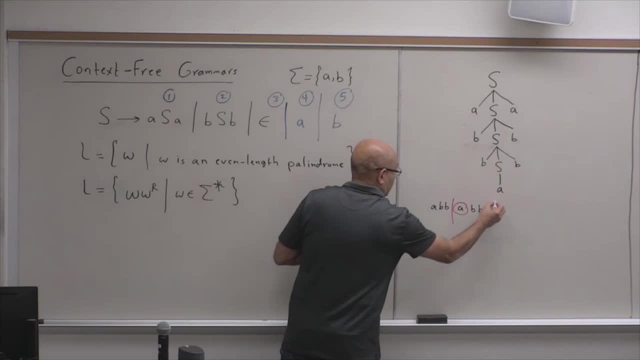 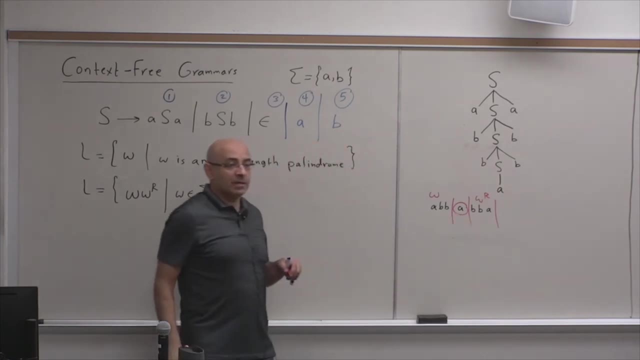 And then this is your W, this is your WR, But in the middle you have some character. Okay, So we change this into a grammar that has five rules. So now it's no longer an even length palindrome, It's a palindrome. 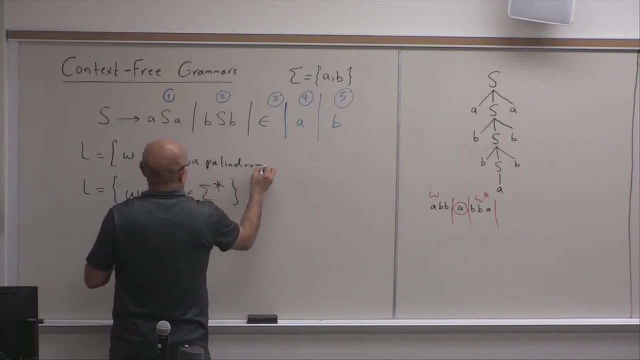 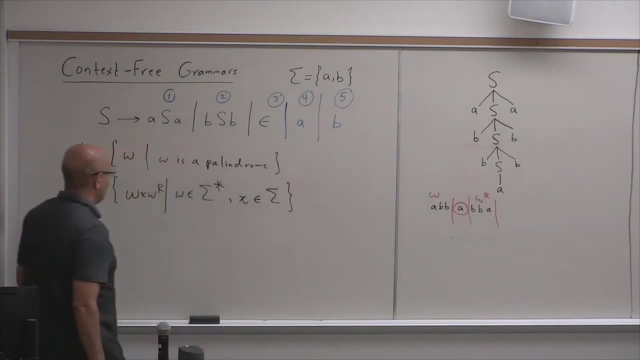 Okay, So how would you modify this? So this is going to be a WWR. W, let's say XWR. That's the W belongs to sigma star And X belongs to Sigma Sigma, Or in fact it should be sigma sub epsilon. 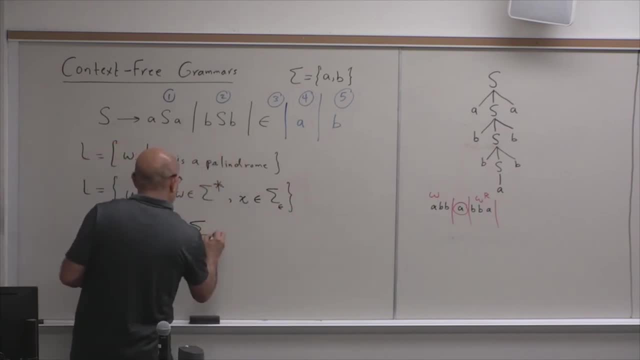 Where sigma sub epsilon is sigma union. Sigma sub epsilon is as we defined for NFAs, is sigma union epsilon. Okay, So in the middle you can put epsilon or you can put any symbol from the alphabet. Okay, Any questions on this? 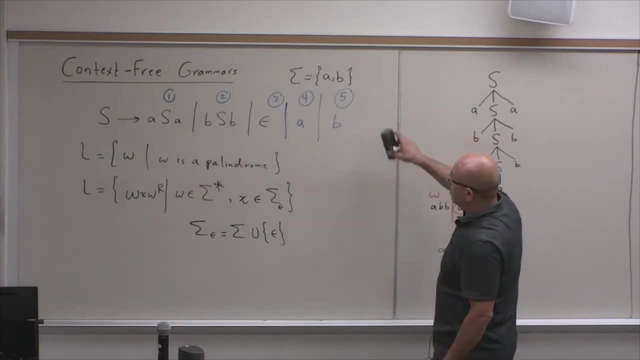 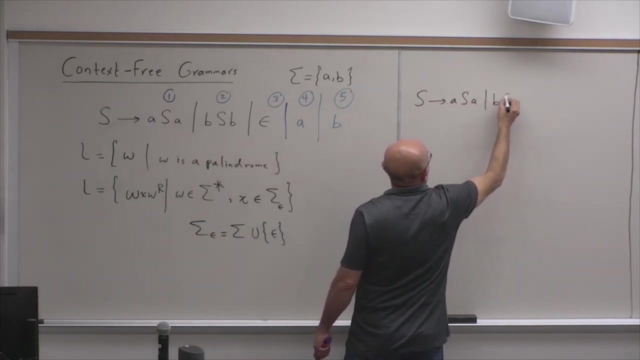 Now I can write, you know, to show you that there are multiple ways. There can be multiple ways for writing a grammar. I can write this grammar as SASA or BSB, Or you know. You know M, Where M is, whatever goes in the middle. 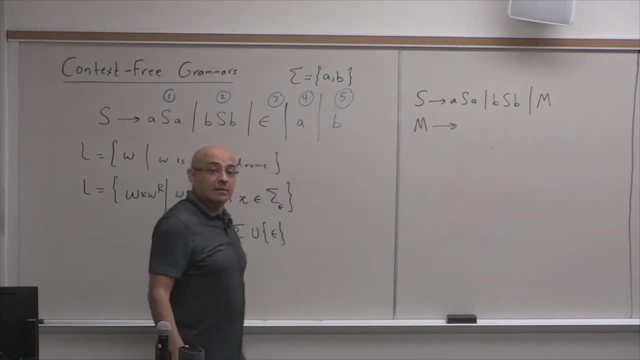 And then I can define M as What's M. So I just took these three options and called them M. So M is just epsilon or A or B. Okay, So this is another way of defining the grammar. This could be a, you know, in my opinion, this is better. 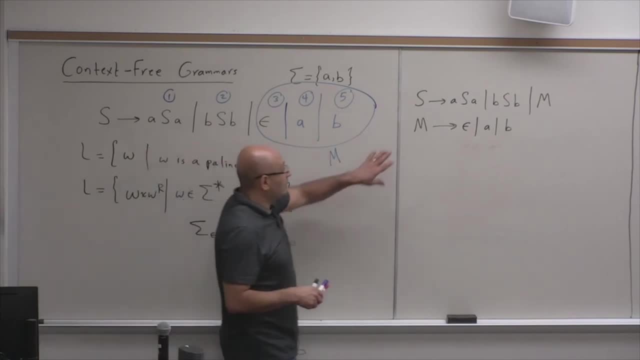 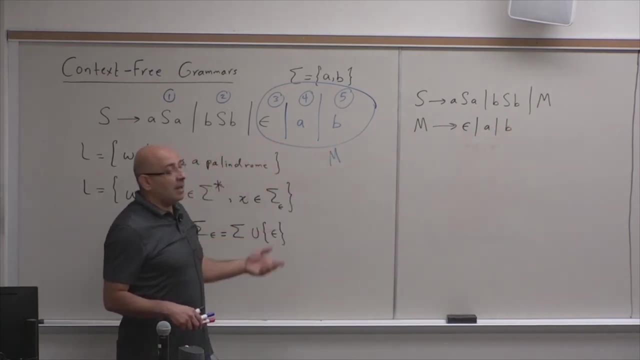 I mean, this is subjective, But yeah, this looks better to me because this is a variable And this variable can be anything, And in fact, you know what if the alphabet has more symbols? So you just you put them here. 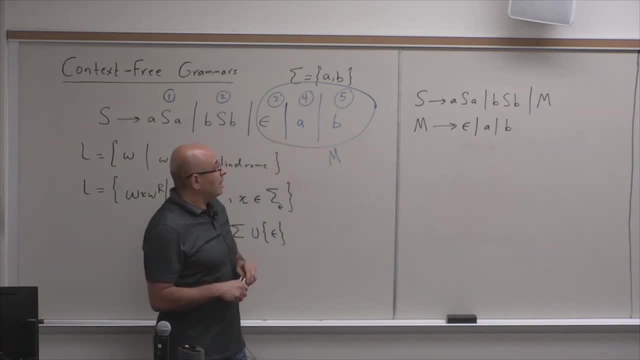 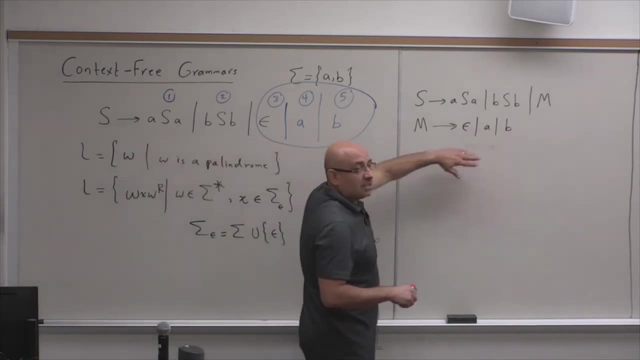 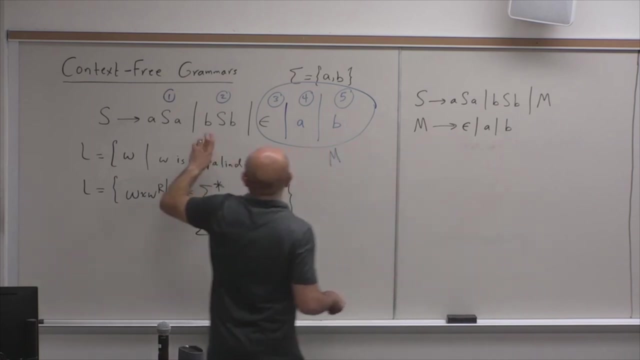 You put them in here And then you can extend this easily. So if you have a C or a D, you can add them, But anyway. So this is just another way of writing the same grammar, So this grammar is equivalent to this grammar. 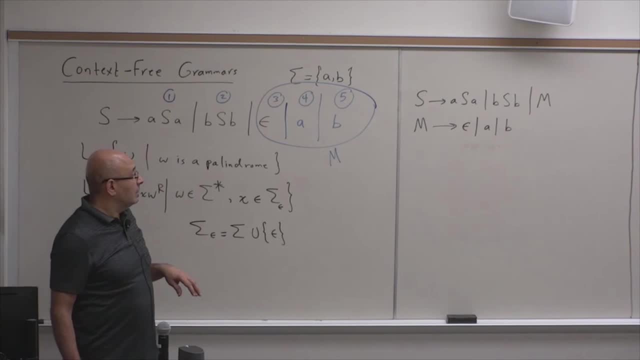 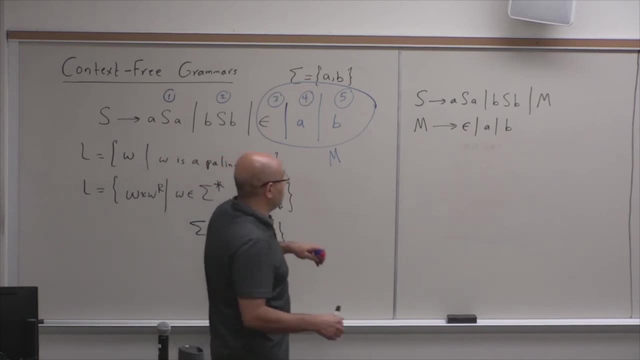 Yes, So if you add another variable, can you still do the S transition with the star? Oh, yes, Yeah, So we can do a derivation like: okay, we can do this, Let's derive. let's derive what.